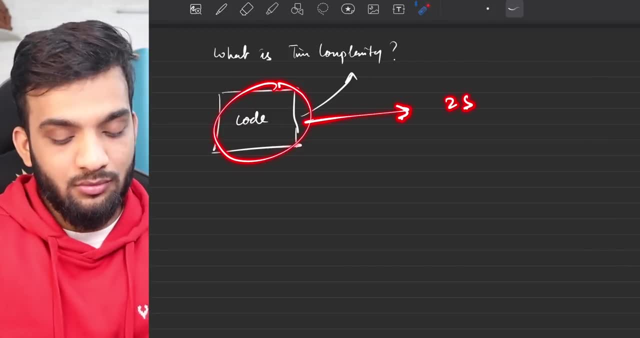 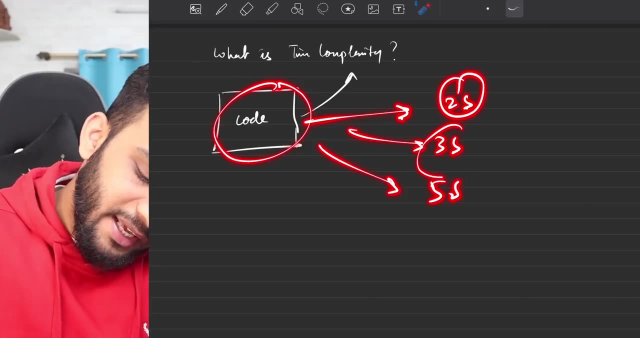 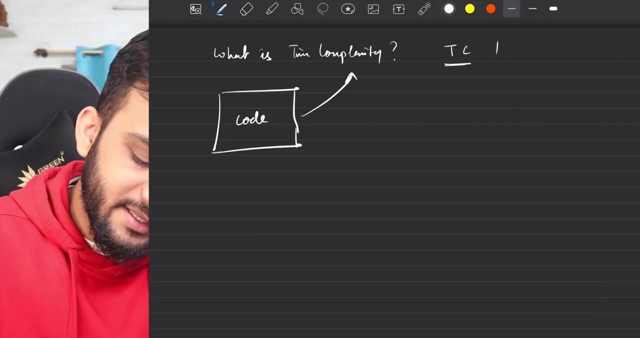 that might end up taking, let's say, two seconds on a machine, or might end up taking three seconds on a machine, might end up taking five seconds on a machine. So the time taken? will you call it the time complexity? No, You will never call time complexity as time taken. Now you might ask: 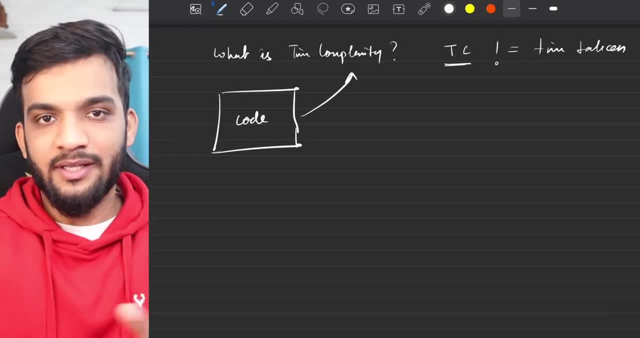 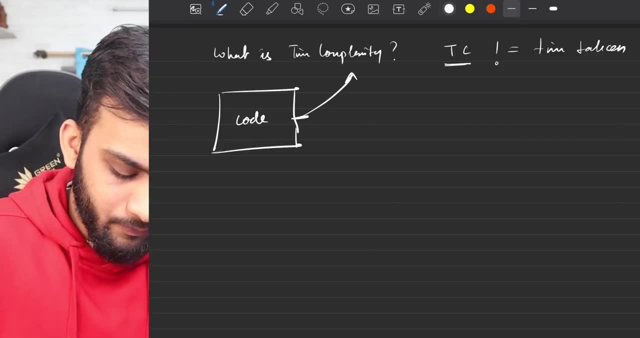 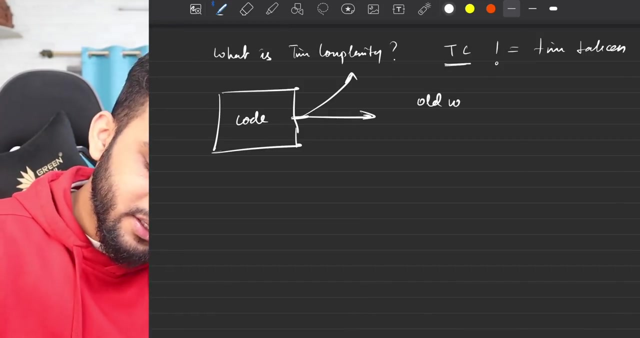 but why? If a code is taking certain time, that should be its time- complexity. Let's give you a very, very easy example to explain why not Imagine: I take this code, I take this code. this can be any code, any code. I take this code and I run it on two machines. One is the old Windows machine. 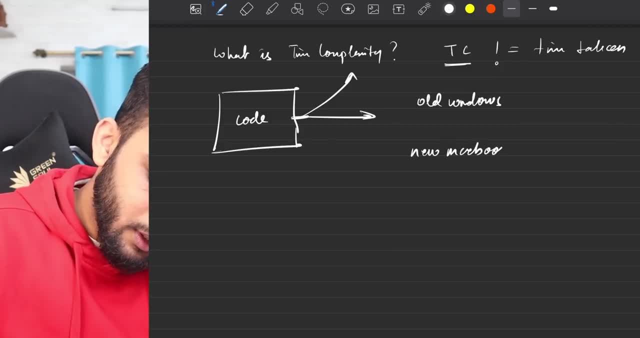 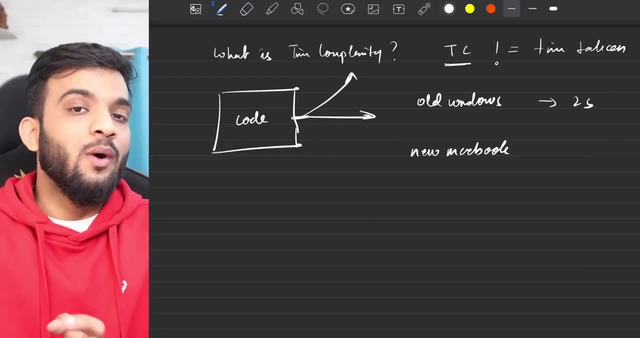 And the other one is the new MacBook machine. Now, I'm sure the old Windows, hypothetically, might end up taking two seconds to run that code. Well, the new MacBook, which is a lot more in terms of the like, a lot more latest in terms of the configuration, 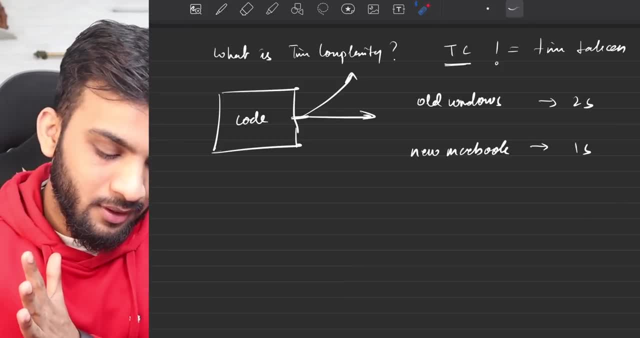 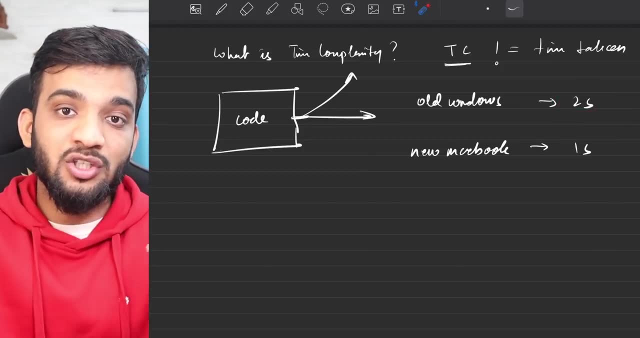 might end up taking one second. So does it mean that your code is taking one second Or does it mean that your code is taking two seconds? It might happen I bring up some other machine the next day. it might end up taking less than one second. So depending on the system, the code, 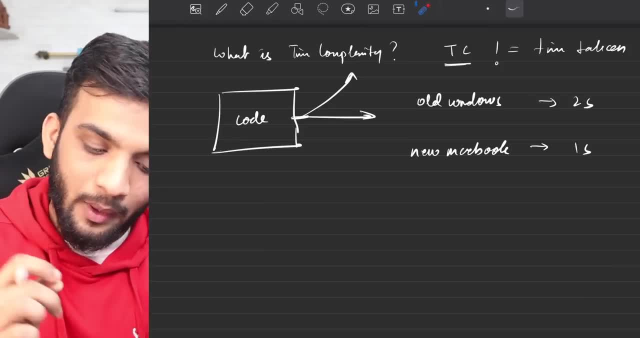 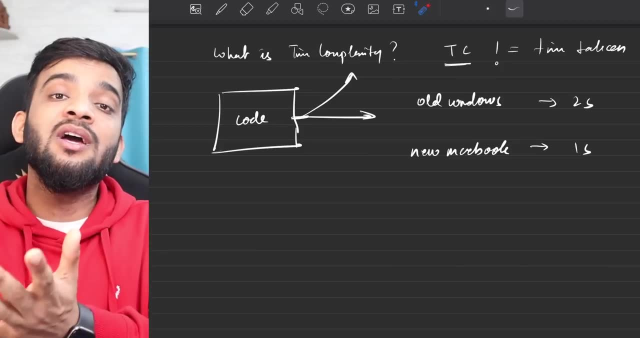 ends up taking a different time. So that is why time complexity cannot be said as time taken, because it is dependent on the time. So it is dependent on the time, So it is dependent on the system. it is different, dependent on configuration, right. so this is why that is. this is the first. 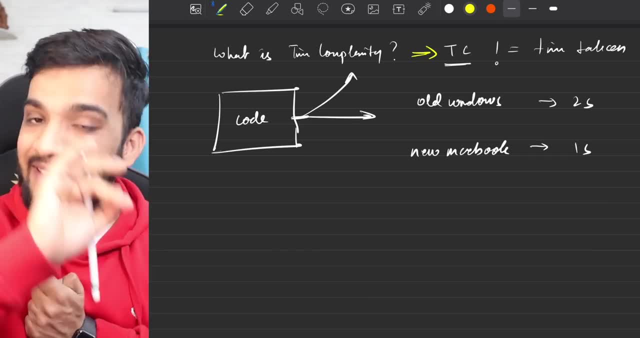 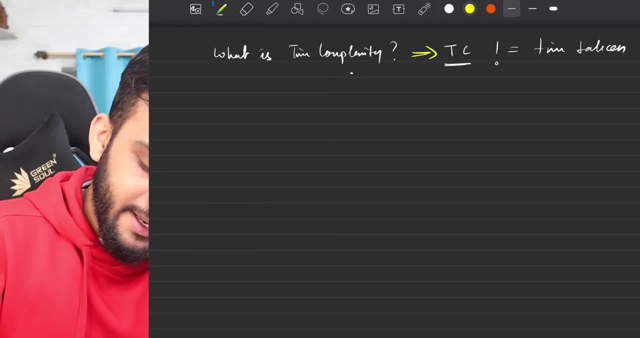 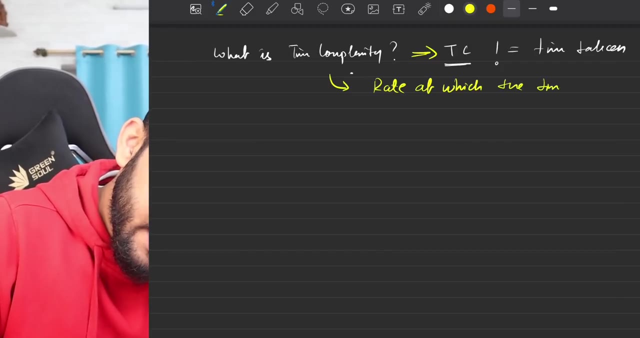 point, time taken is never equal to time taken. never, ever. so, you might ask, if time complexity is not time taken, then what is it? that is where i see the definition: the rate. remember the rate at which the time taken increases, the rate at which the time taken increases with respect to 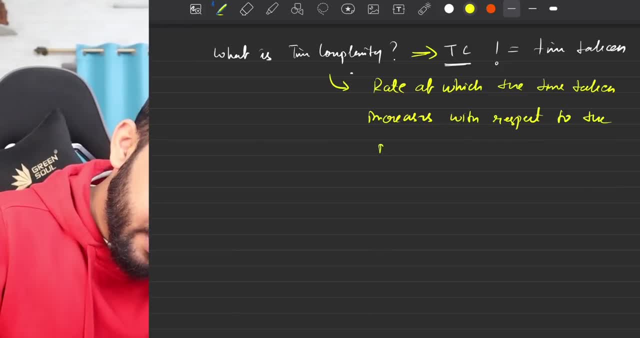 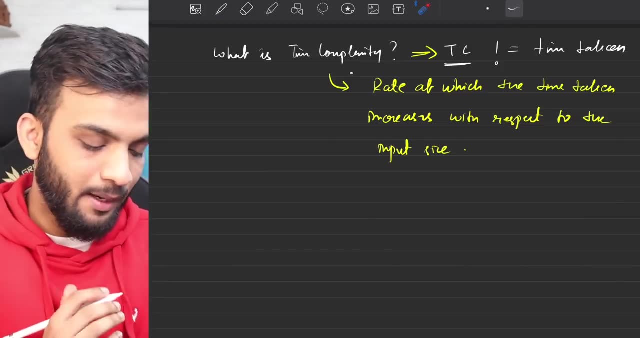 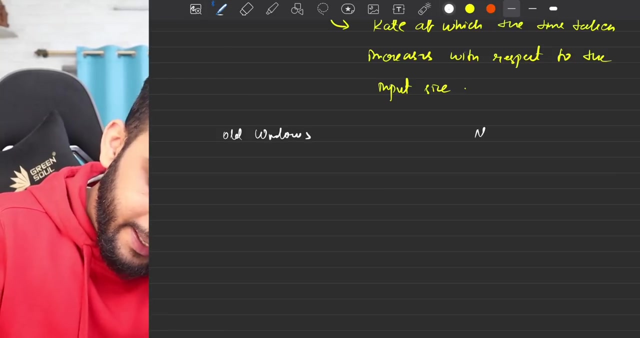 the input with respect to the input size, rather. so what does it mean? let's explain this with the help of a graph. so again, let's take the same example where i'm saying: i have a old windows machine and i have a new macbook. okay, now imagine you're giving the old windows a size. 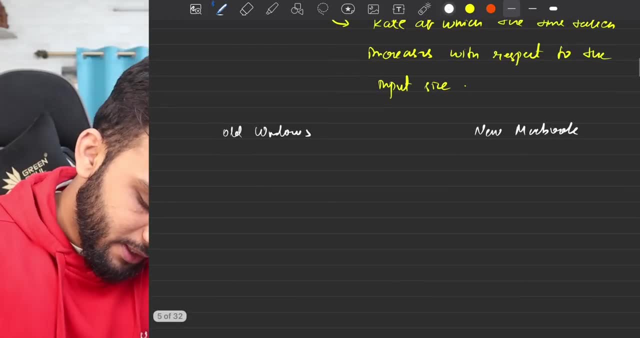 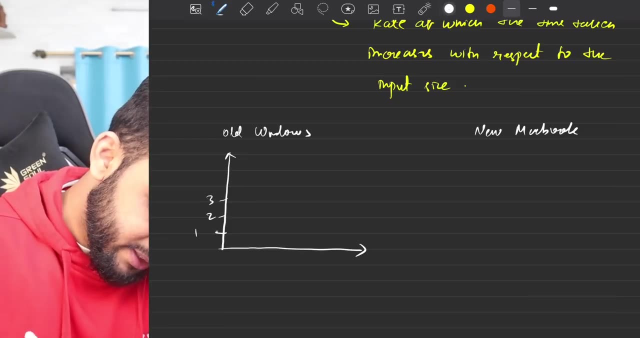 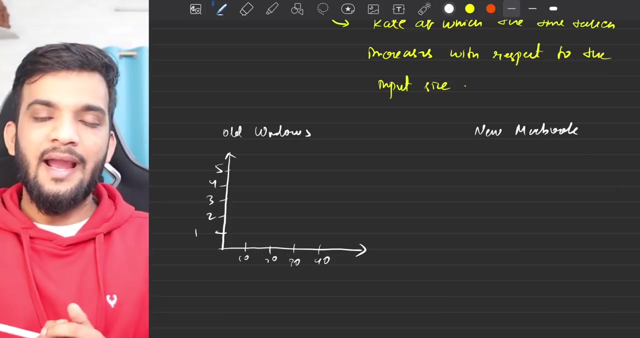 10, just as hypothetical a size, 10 input size, and i'm plotting the graph: and this is one second, this is two second, this is three second, this is four second, this is five second. this is 10 input size, 20, 30, 40.. at 10 input size, it might end up taking two seconds. 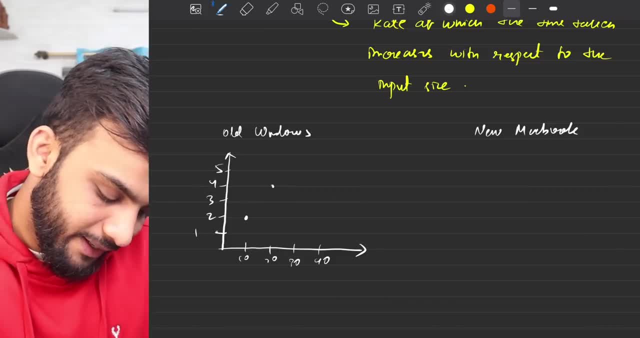 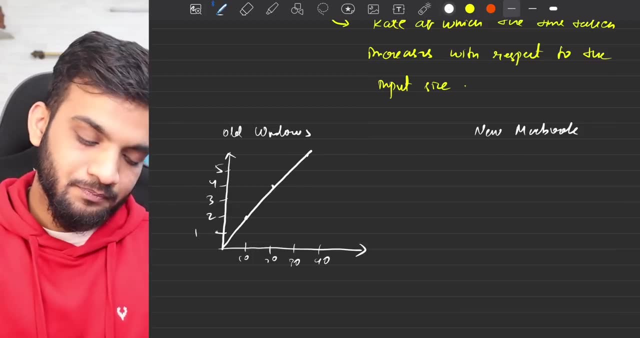 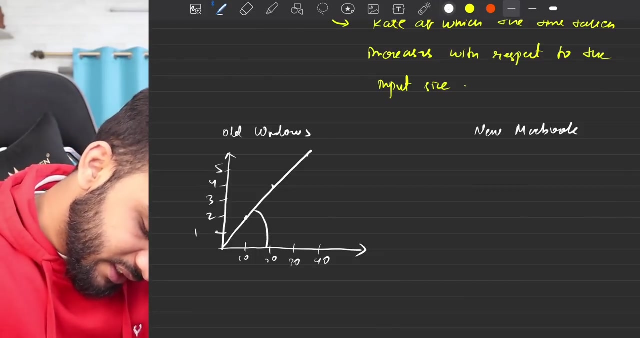 at 20, it might end up taking four. at 30 it might end up taking six, which will be here. so you see the time increasing at some, at some theta angle, like it's increasing at a certain slope. so this increase, this increase, this theta angle is what you call as the rate of increase. 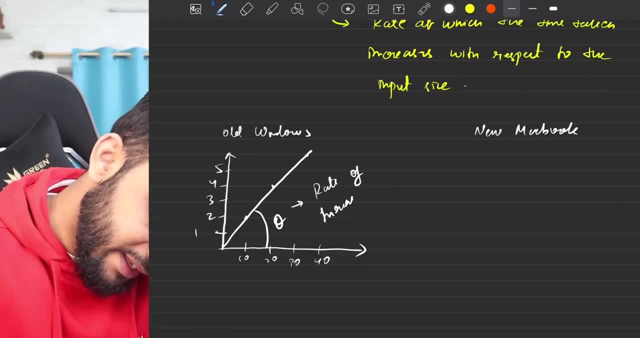 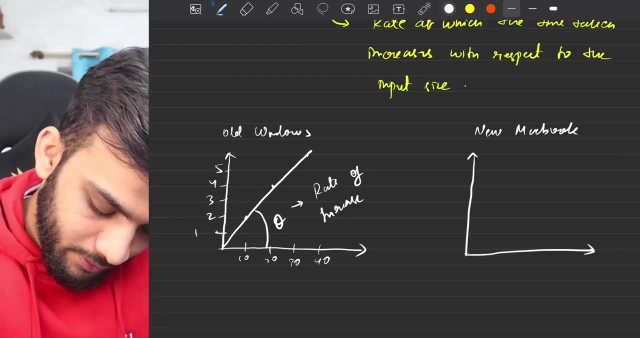 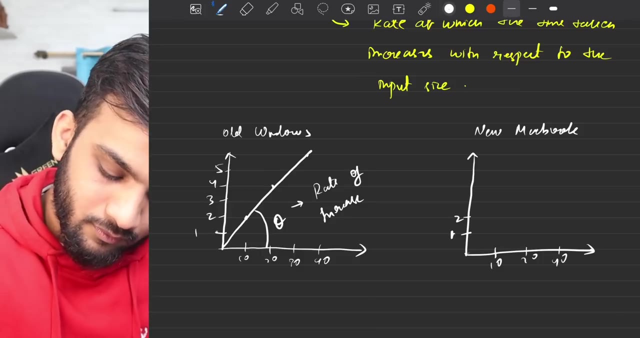 this is what you call the rate of increase. okay, now let's see the new macbook. so if i take the new macbook, the 10 might end up taking one second, the 20 might end up taking two seconds, the 40 might end up taking three seconds. so it's here, here, here. so this is the rate. 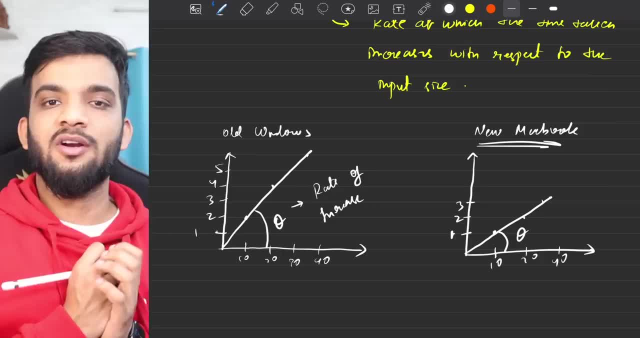 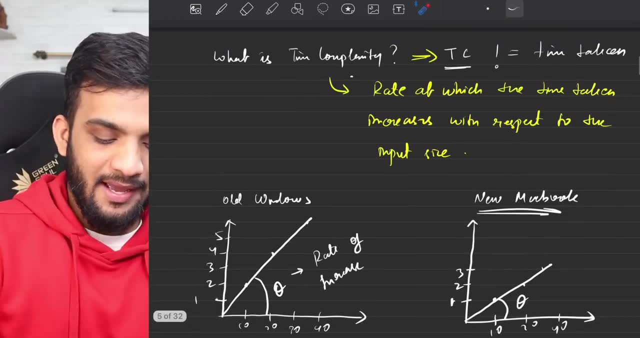 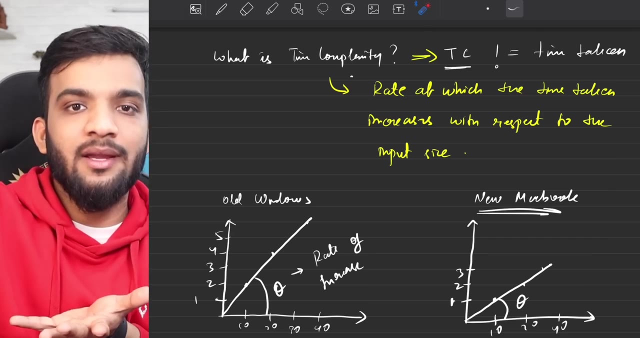 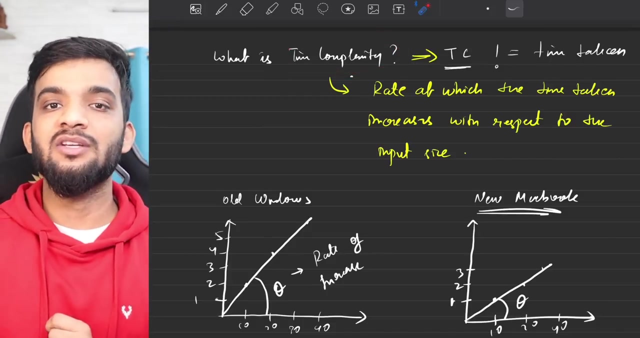 and this theta is the rate for the new macbook. so i can say the rate at which it increases time is what you call as time complexity. on input, if they are giving you more input it might end up taking a certain more time. so the rate at which the time increases is what is generally referred as time complexity of any 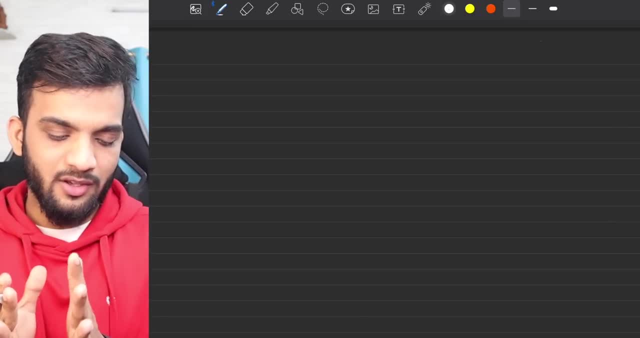 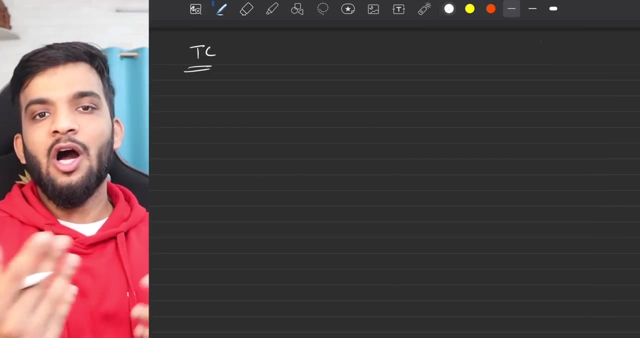 given code. the next question that might come to your brain is: okay, striver, if we are saying the time complexity is not computed in terms of seconds or minutes, then how do we? how do we write it? this is where something like a big oh, a big o notation comes in. 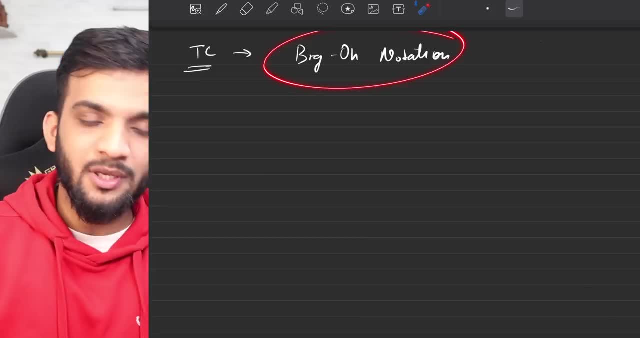 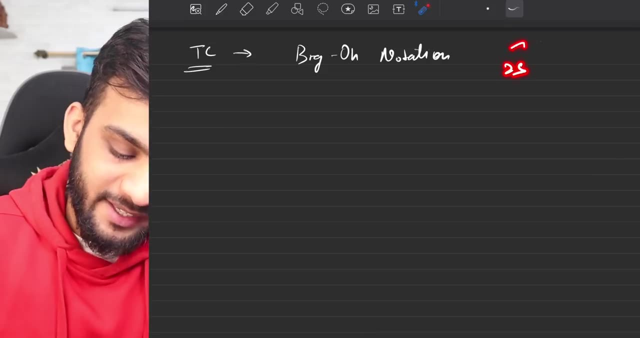 now, in all the interviews that you're going to give, or in all the examinations, if you're writing a piece of code, they will ask you to analyze the time copy. that is when you do not like. you will not say two seconds, no, you will say it in terms of bigo. 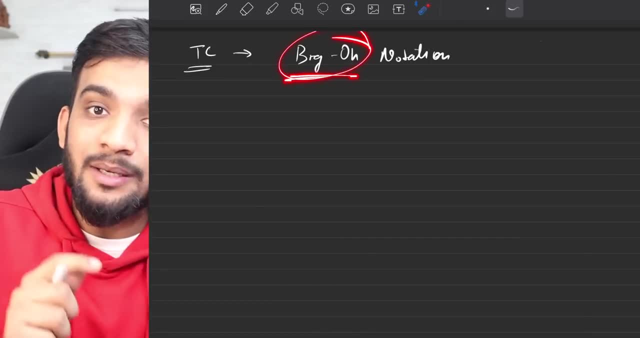 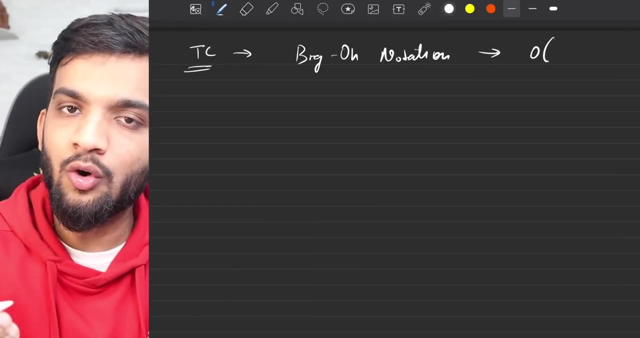 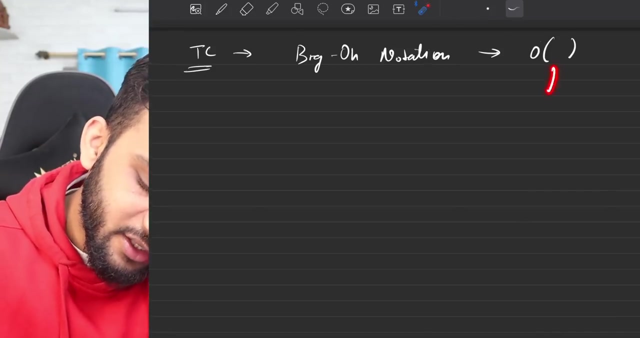 notation. every piece of code takes time in terms of bigo notation. what is bigo notation? i'll just give you a prime example. so it's like a capital o open parenthesis and a close pattern. this is what bigo notation is and inside it you write whatever the time is taken. inside is you write the time. 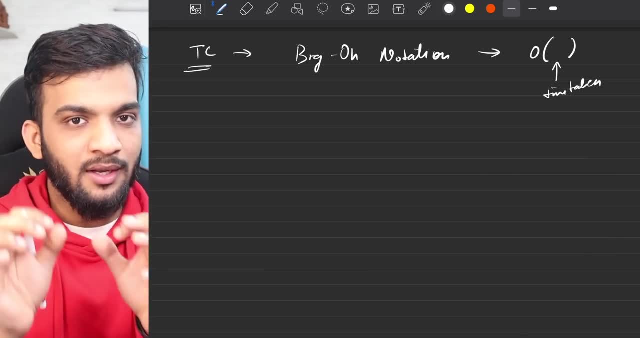 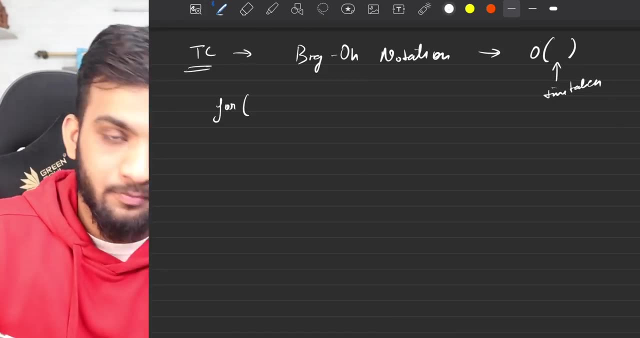 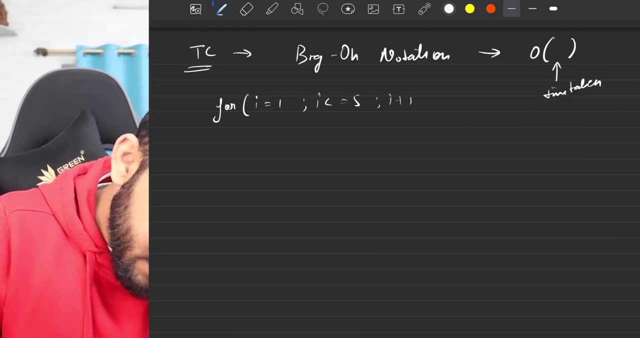 taken, or the hypothetical time, which i'll show you how to compute. let's take a very, very small example to compute the time complexity of a certain code. so imagine i write the for loop. i've already taught you loops in the previous video. i equal to one, i lesser than five, i plus plus. 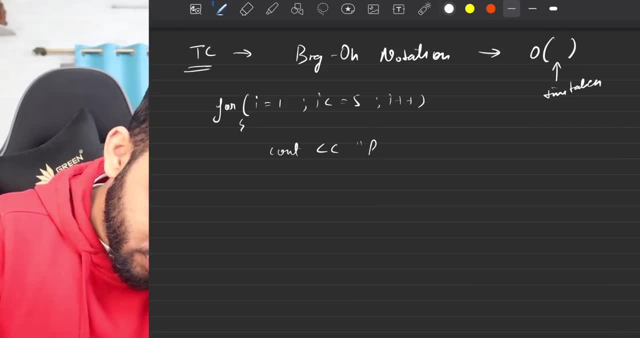 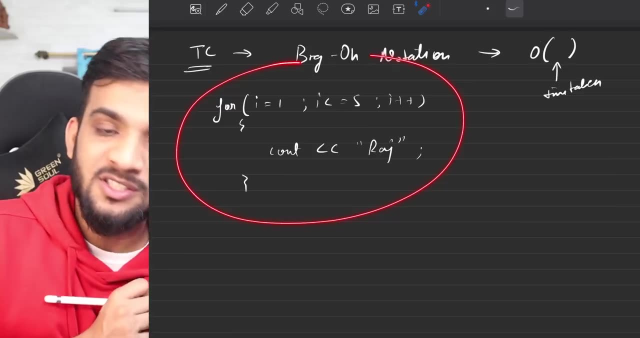 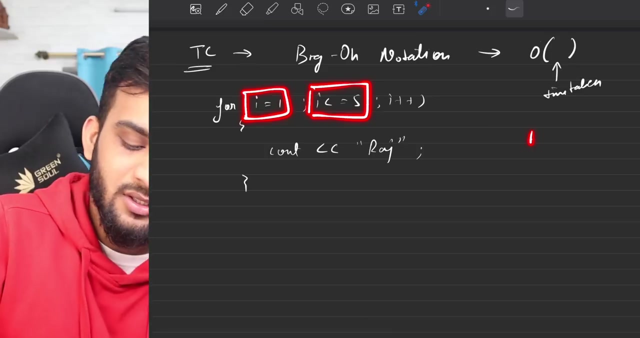 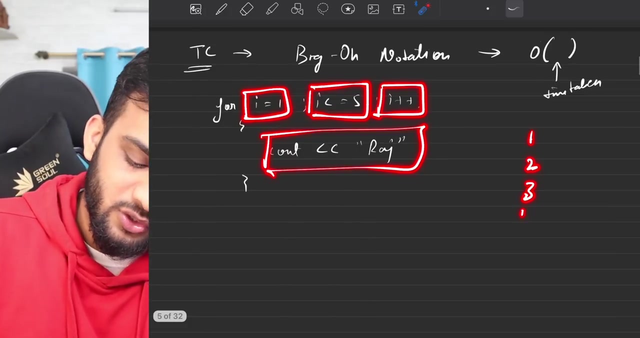 and then i write c out and my name raj, okay. so can you tell me? what is the bigo of this? this is nothing, but the number of steps that this code will take. first step is very short: assigning. the second step is comparison. the third step is printing right, and then you come across, and this is your fourth step. 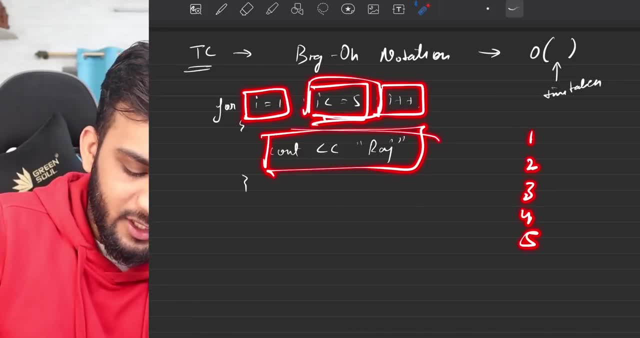 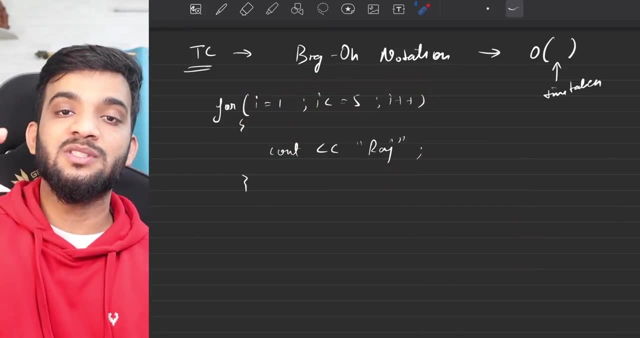 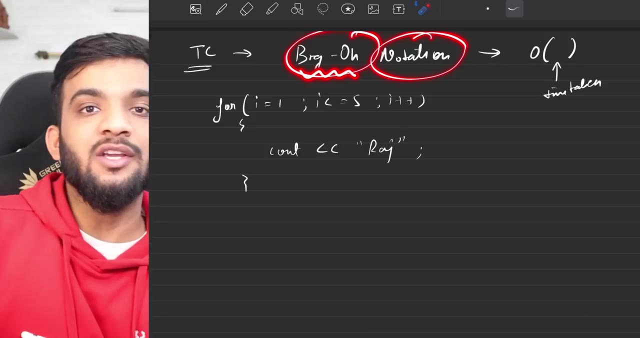 and then again you check: this is your fifth step. and then again you print: this is your sixth step. so this is how every step is computed. so whatever is the total number of steps, that is what you write inside it and that is what you call as the prime bigo notation. but you cannot just keep on counting. 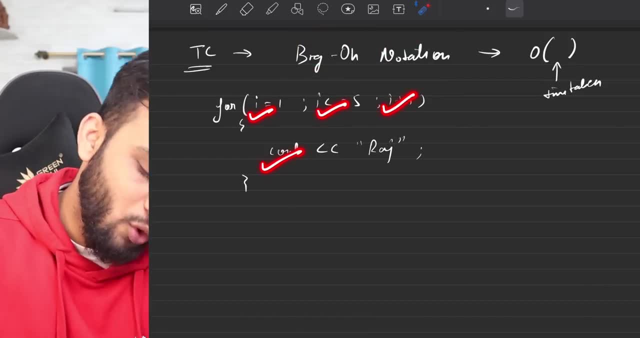 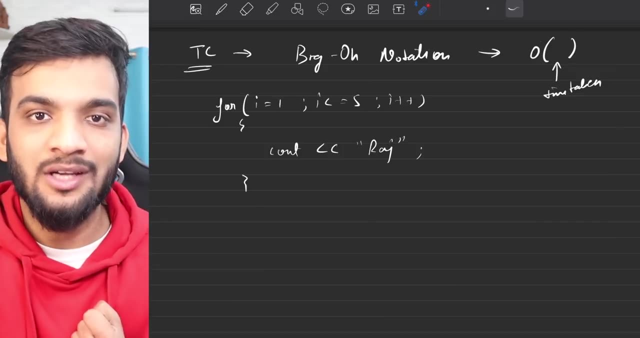 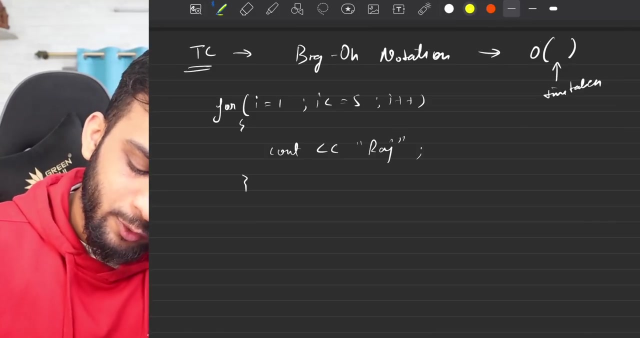 step one, step two, step three, step four, step five, step six, step seven. that is insane. you just cannot keep on manually counting the steps. this is where three rules come in and i'll write the rules, the rules. the three rules are very simple. always compute time, complexity in terms of worst case. 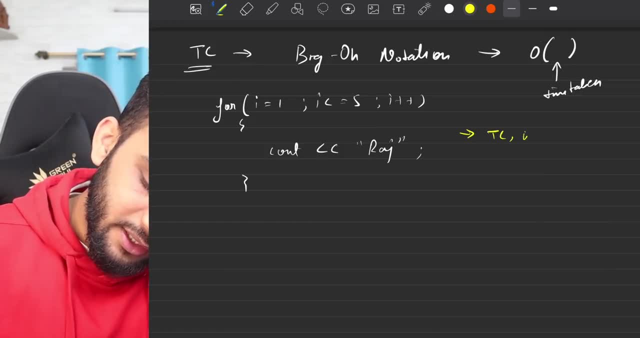 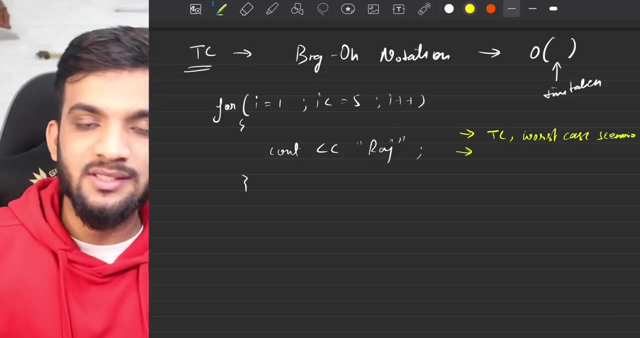 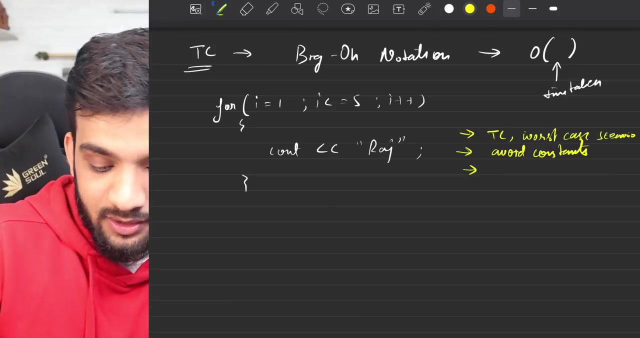 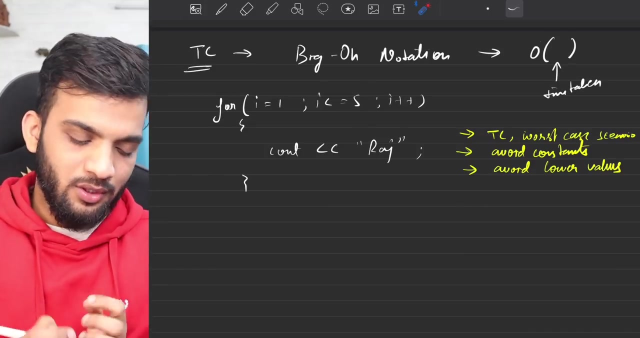 scenario: time complexity to be computed in terms of worst case scenario. why worst case? i'll explain you. the next one is: avoid constants. avoid constants. the third and the third is: avoid lower values. so if i have to compute the time complexity or the bigo of this piece of code, 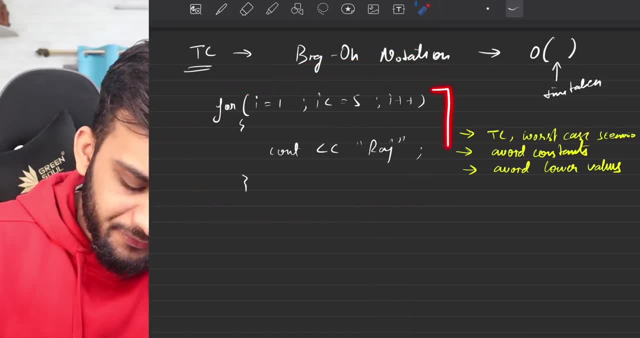 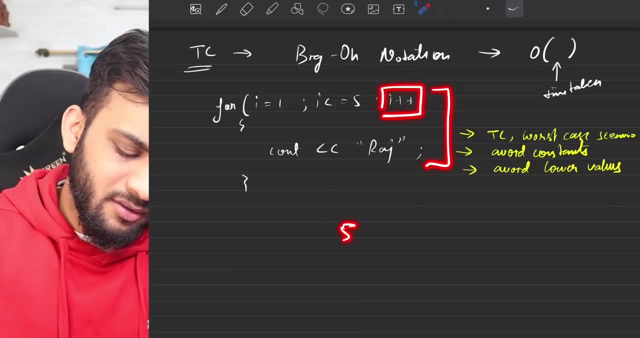 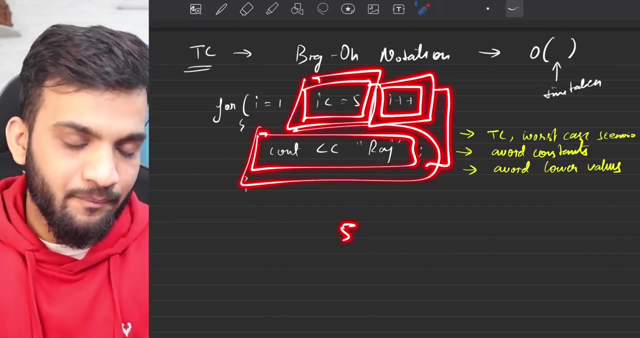 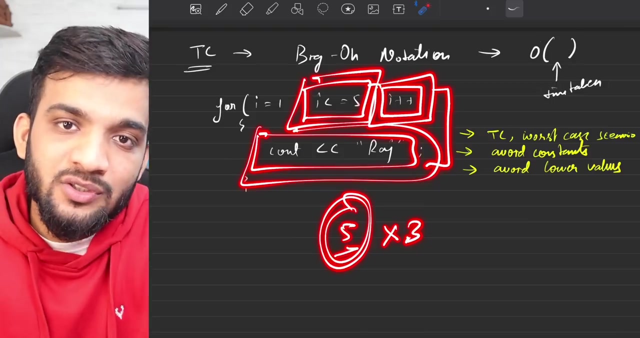 let's look at it on a very high level. can i say this: for loop is running for five days, i can at every time what is happening? it's like increment check print, increment, check print. so can i say: for every time it's all operating twice. for every time it is operating three times. increment check print five into three. 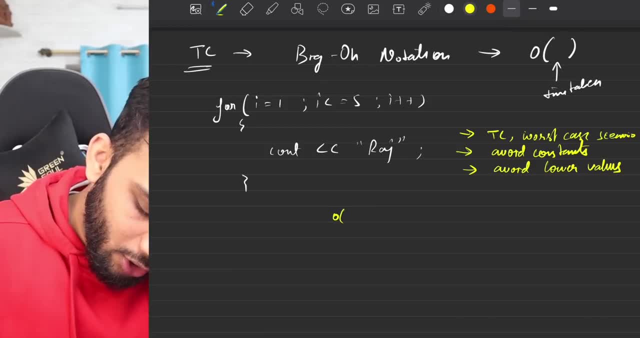 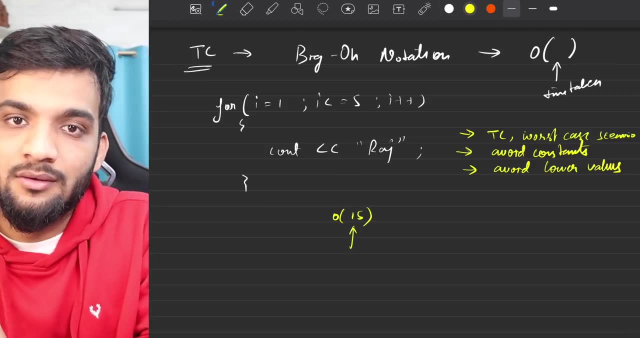 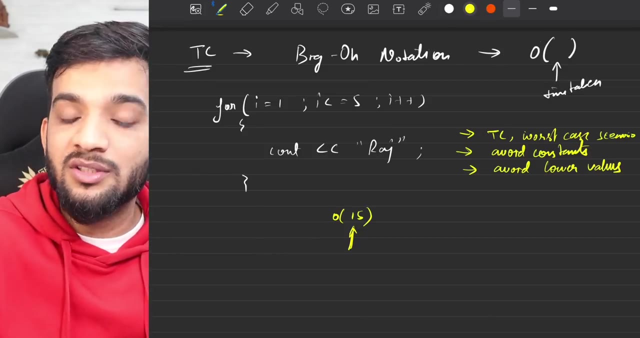 can i say this? i can, so can i say a total of 15 times? that is how you write it. you write it as bigo of 15 is what you write, and this is time complexity. it runs for 15 times, but this is a number. this is a number. you generally do not represent your code in terms of numbers. okay. 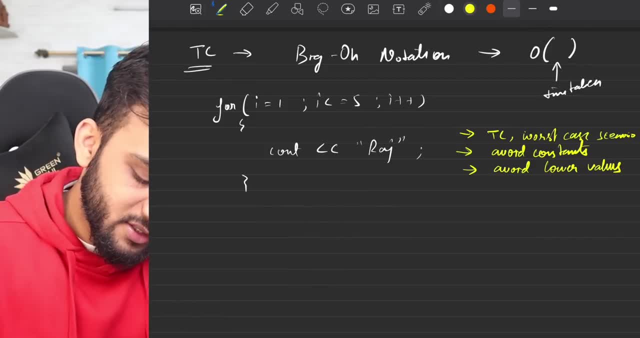 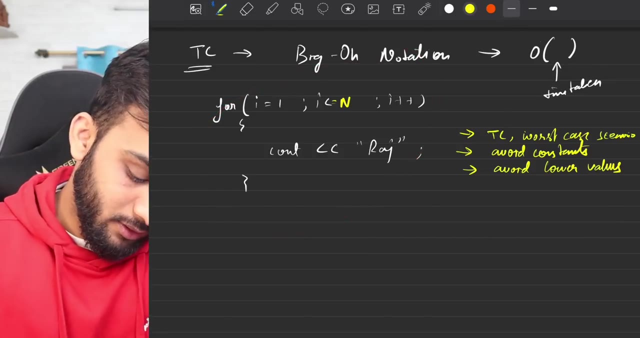 so let's, let's change this now. can i say this: if i change, uh, this demand, if i, if i probably will change this to lesser than n, less than equal to n. so now can you say how many times will this loop run? i know one thing: this is going to run for bigo of n times the loop. 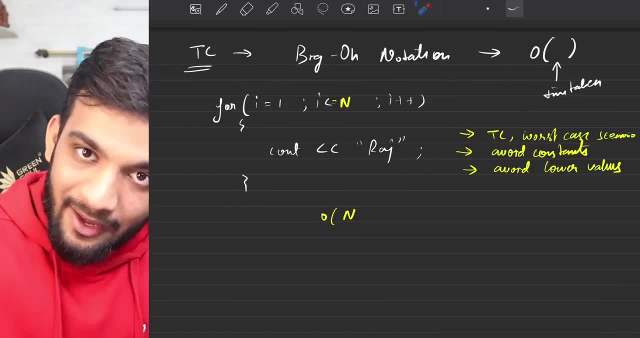 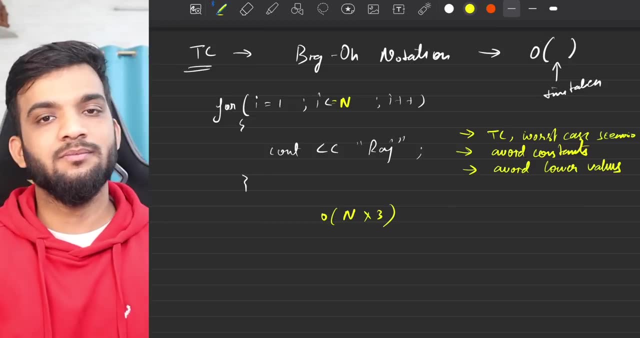 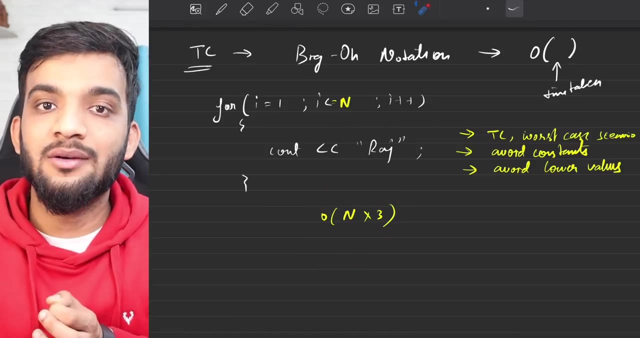 the code will run for n times, n iteration, and at every iteration, one, two, three things will happen. that every iteration, three things will happen. very obvious. this is what will be the time: complexity we go off n. we go off 3n will be your time. so whenever you're saying b go, you go to the code. 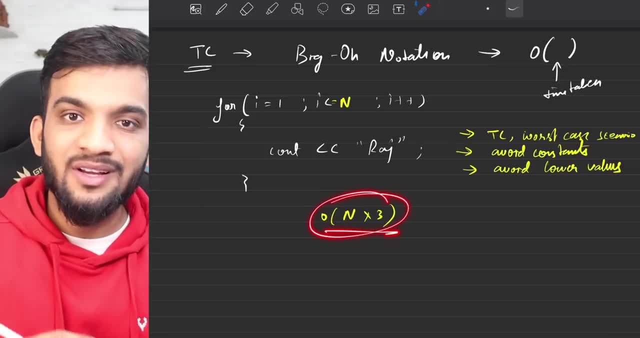 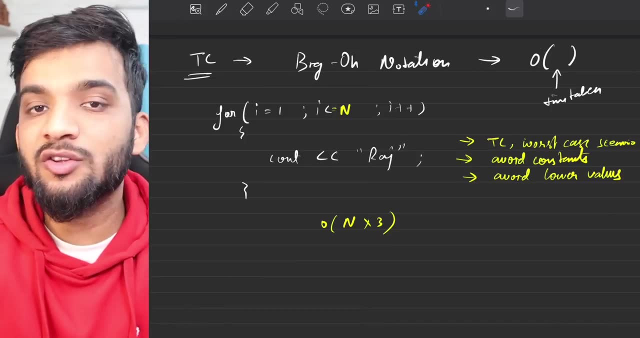 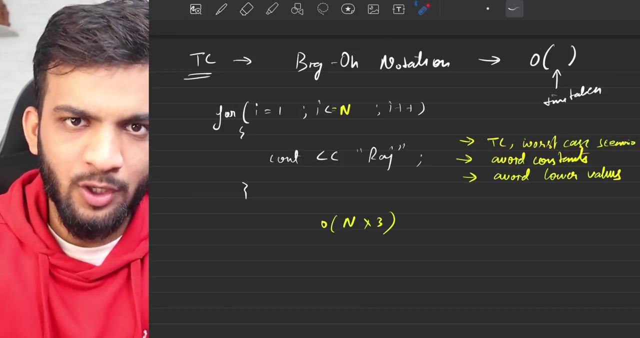 and you see how many times it is running and then you write b, go off 3n as your time complexity. does that make sense? it does right. okay, let's now come back to the three points that i've written. always compute time complexity in terms of worst case scenario. now there are three things. one is the best case. 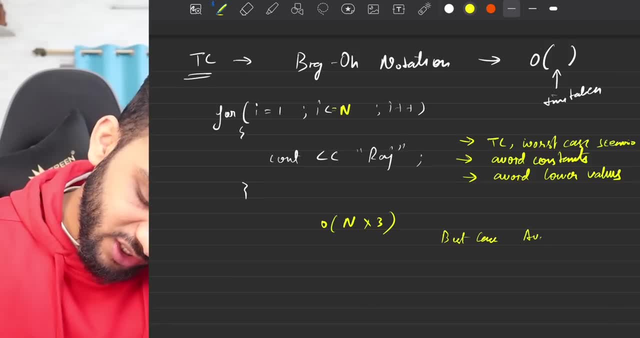 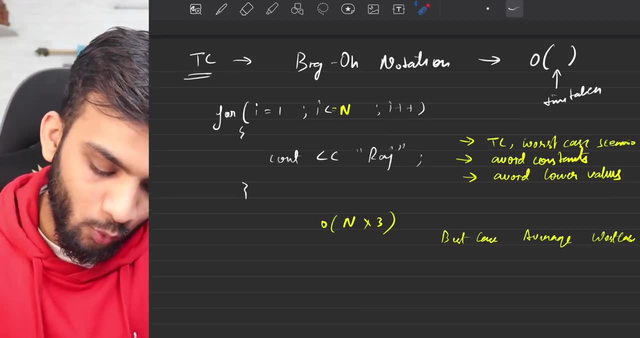 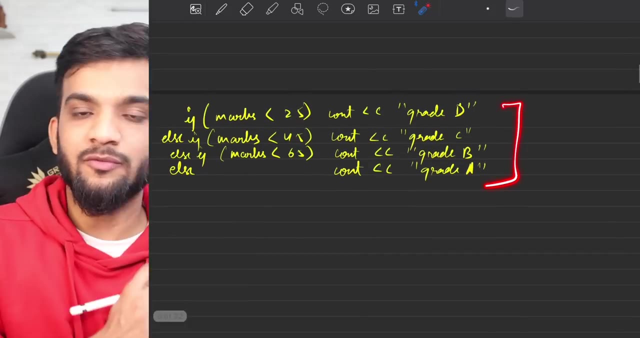 one is the average case and the other one is the worst case. now let's take a snippet of the code and explain you what is best case, what is average case and what is worst case. okay, let's. so this is the snippet of the code. now imagine. the snippet of the code is very simple. it states: if marks is: 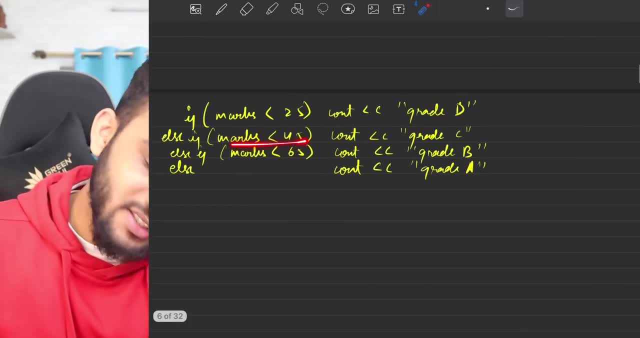 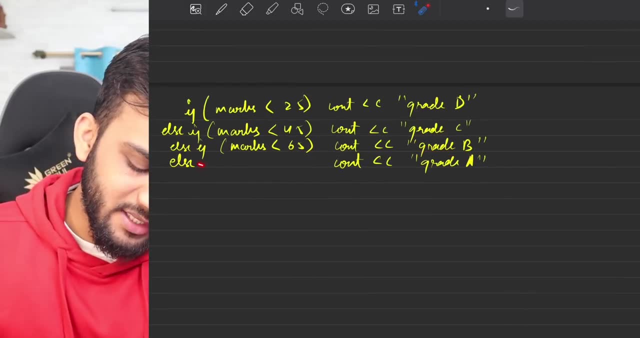 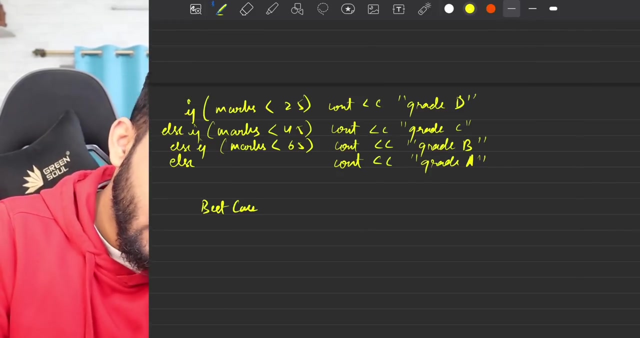 lesser than 25, print grade d. it states: if marks is less than 45, print grade c. if marks is lesser than 65, then you go ahead and print grade p, or else you go ahead and print grade a. so let's talk about the best case scenario. what is best case? when the program takes the least amount of time. 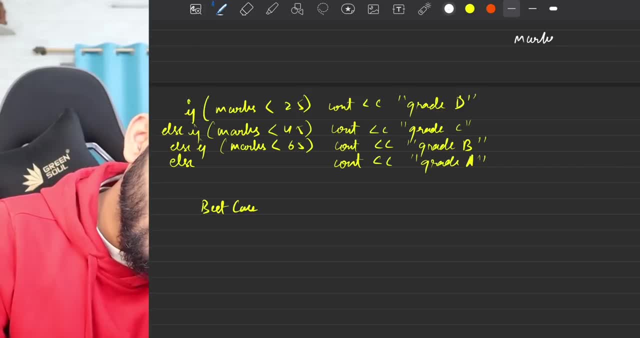 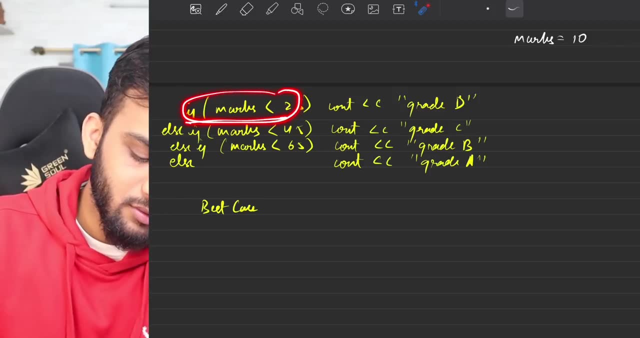 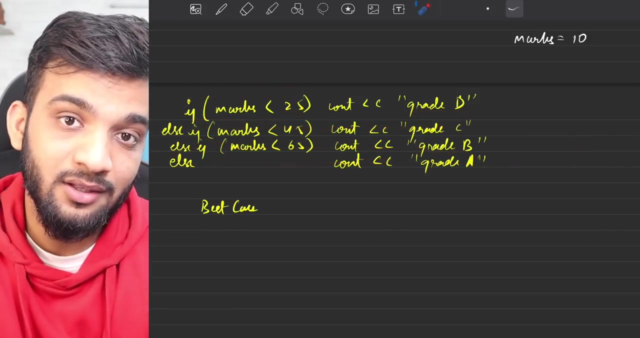 so over here, can i say: if someone gives you an input of marks equal to, let's say, 10- 10, what will happen? this will execute it and grade d will be printed and none of these lines will be executed. none of these lines. so can i take? can i say the number of operations will be just one. 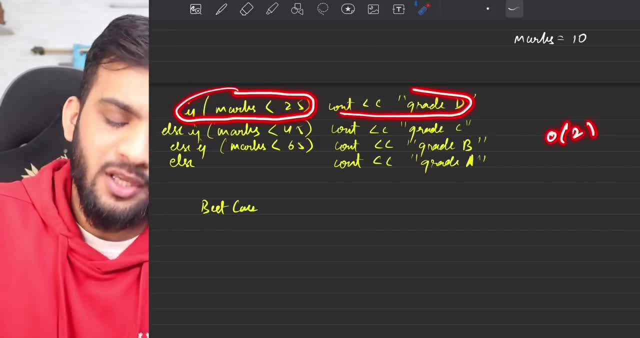 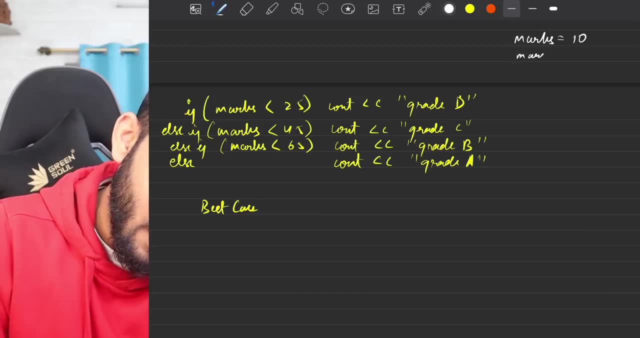 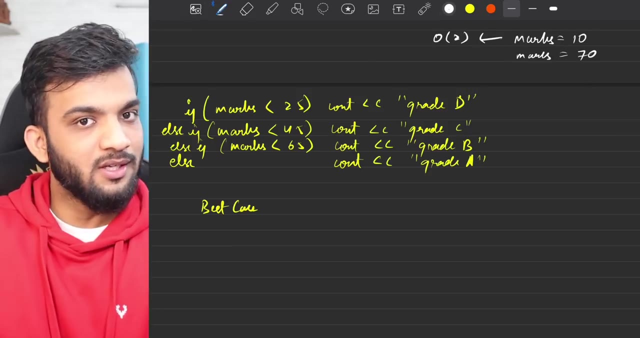 a check and a print which is like two operation. which is like two operation. can i say: imagine if i give you marks equal to 70, so at marks 10 it was bigo of 80 operations, correct? we go of two operation. now if i give you marks equal to 70, what will happen? 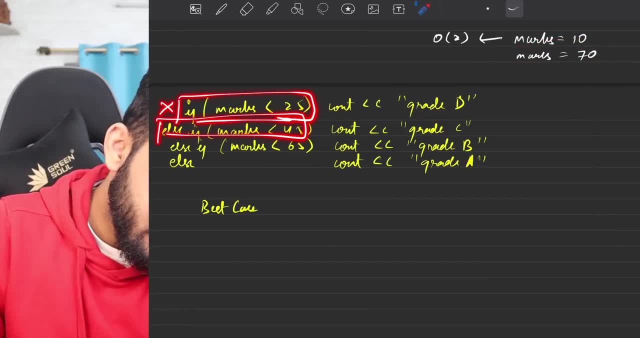 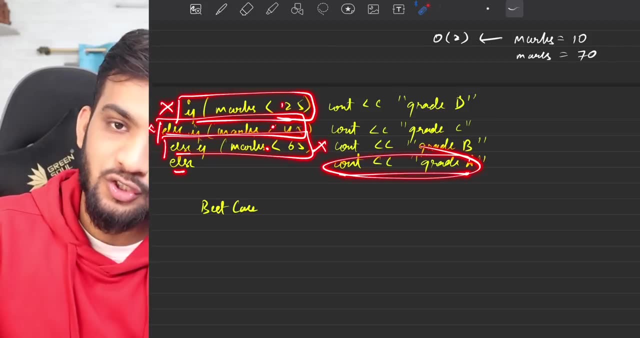 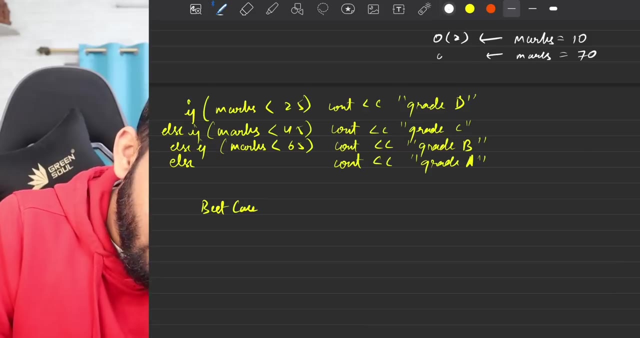 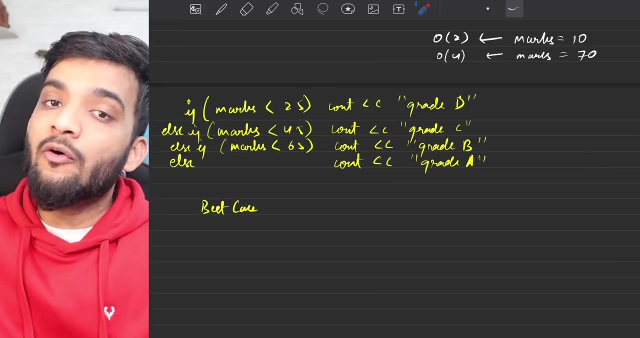 check, false, check, false, check, false. it comes here three and then four. can i say four operations were here, like one, two, three and then goes to else somewhere around four operations. so it takes four operations. so whenever you're analyzing the time complexity, will you say: say that my code runs in b go 4, or will you say that your code runs in b go 4? obviously you will. 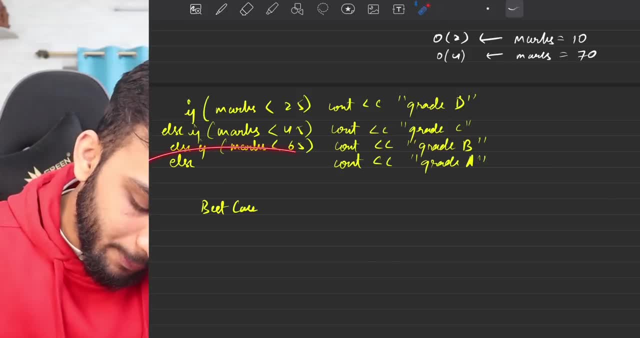 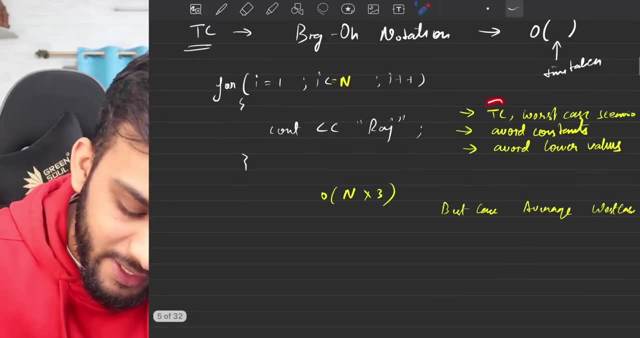 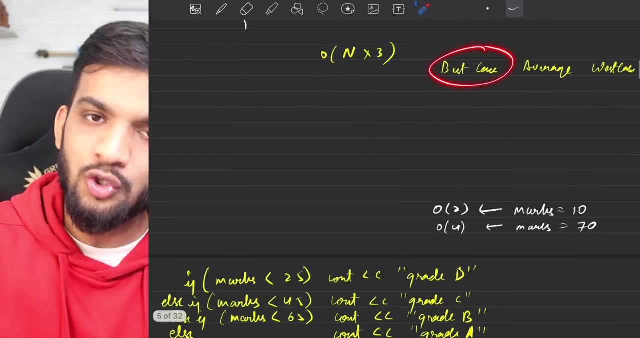 say b, go 4, because that might be the worst case that the computer might encounter when it is given an input. so always, yes, always- compute the time, complexity in terms of worst case scenario and if they will ask you the best case, you know the best case. whatever is the best case, like in this. 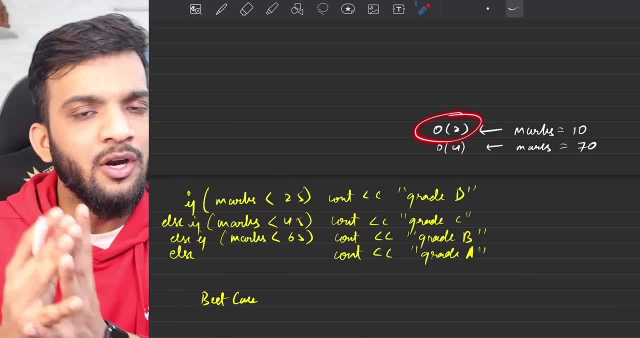 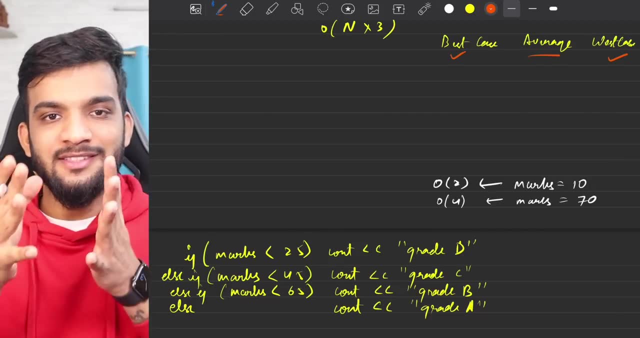 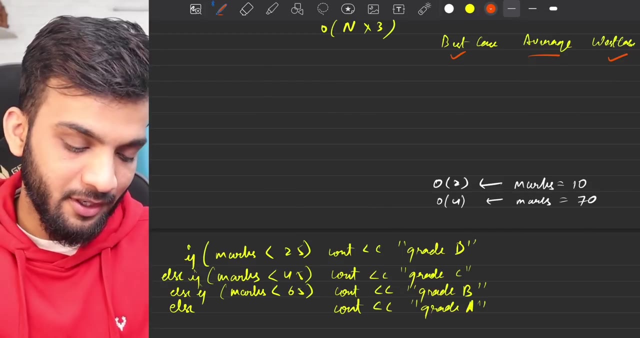 case is the first if statement getting executed, which is b go of two operations. so you've got an idea about the best case and the worst case. you know what is the average case? there's nothing but the best plus worst, and divided by two, it's it's the median of it. so pretty self-explanatory why. 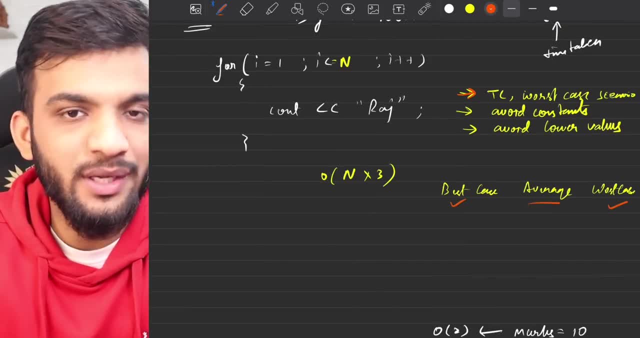 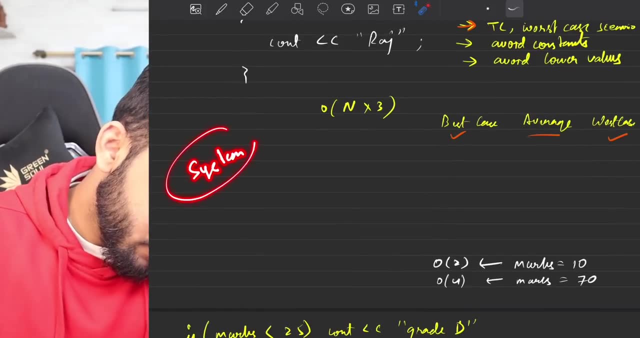 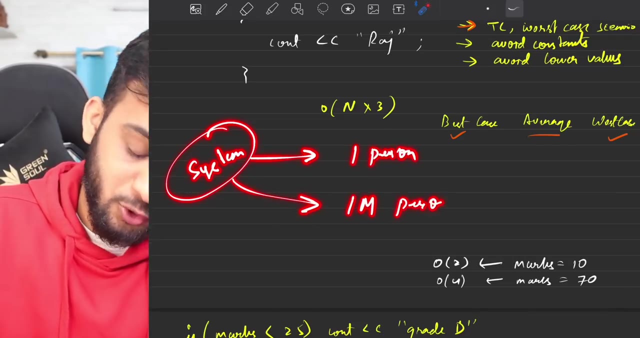 if i give you a question, why do we compute it in terms of worst case? the answer is again self-explanatory. if you're building a system, will you build it for one person, or or will you build it for one million person, if given an option? 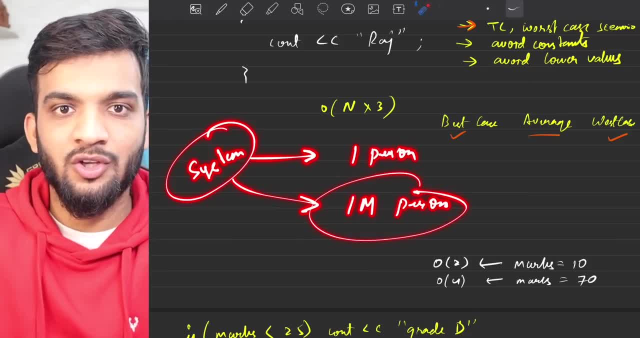 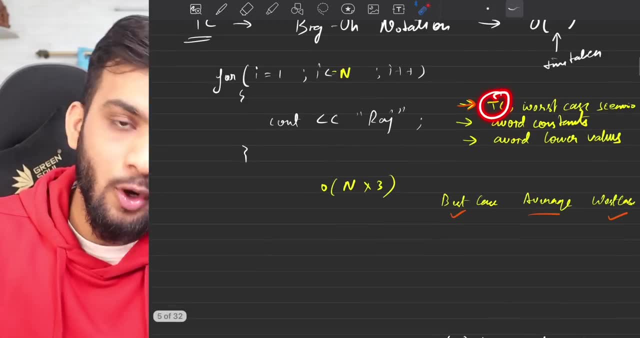 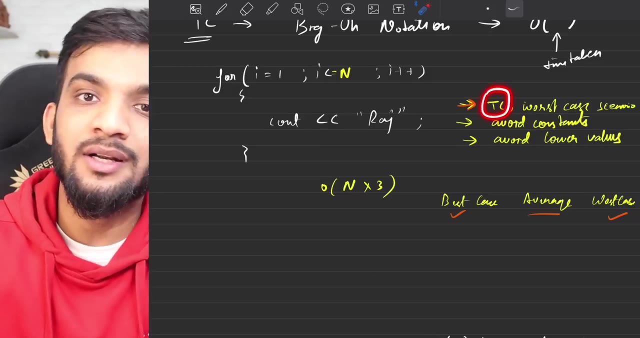 if, given an option, you will say one million, because you want to build a system which can scale up. you always think of the worst that can happen. that is why, when i talk about time complexity, your code's extreme, worst case is what is considered while computing time complexity. 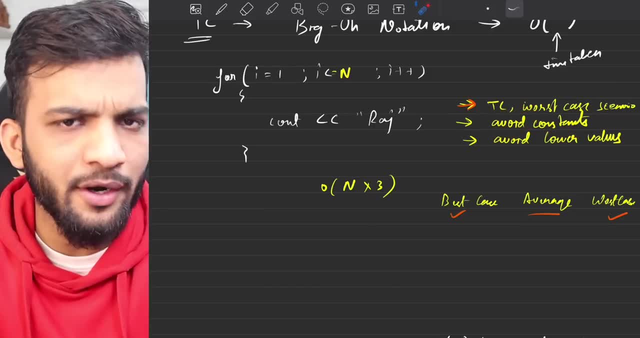 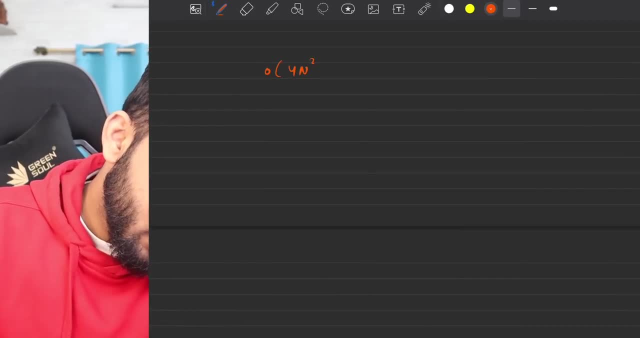 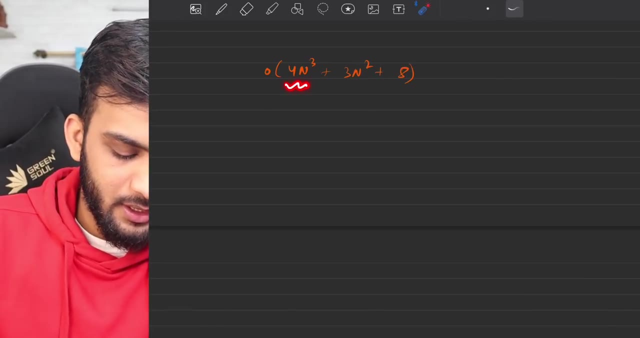 now let's talk about constants. i'm saying: avoid constants. why am i saying that? let's take a shuttle example. let's take something like 4n cube, something like 3n square plus 8. let's take this. so over here: 4n cube plus 3n square plus 8. these are the number. 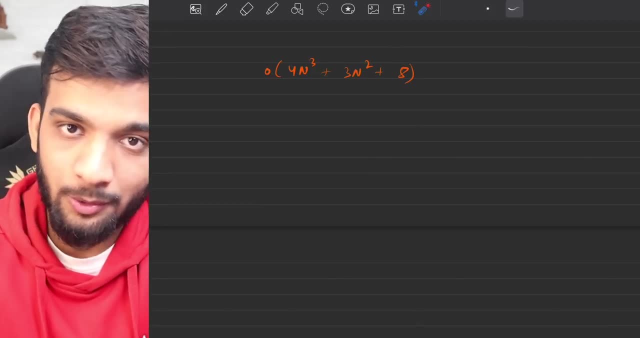 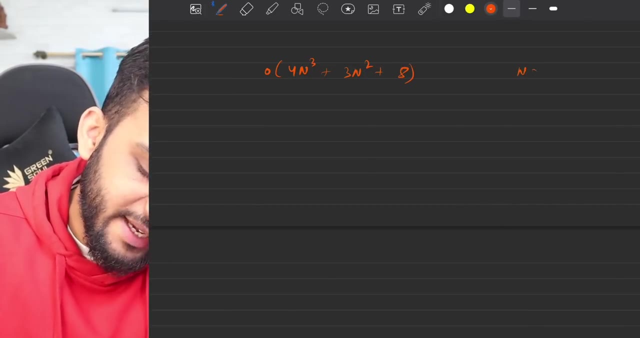 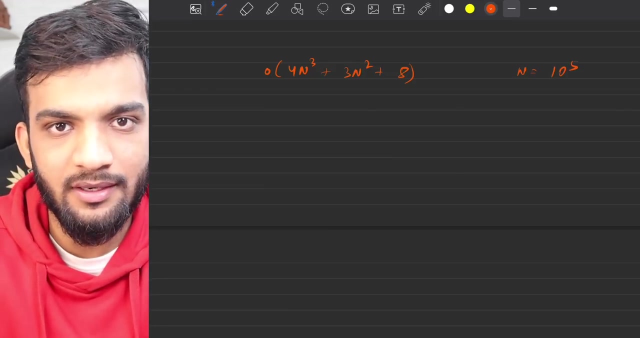 of operations that your code is taking hypothetically. i do not know the piece of code, i'm just taking a hypothetical we go expression. now imagine if i tell you that the input size n, the input size n, is somewhere around 10 to the power 5. right, i'm saying 10 to the power, 5 is the input size. 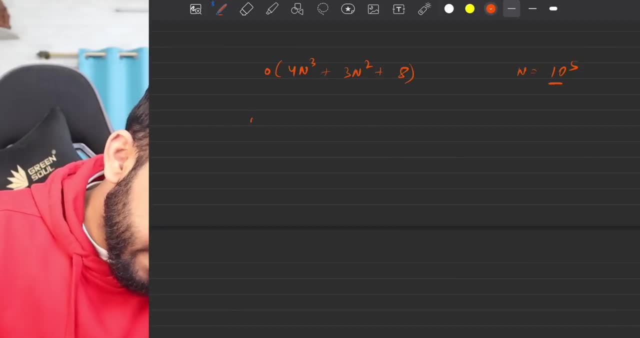 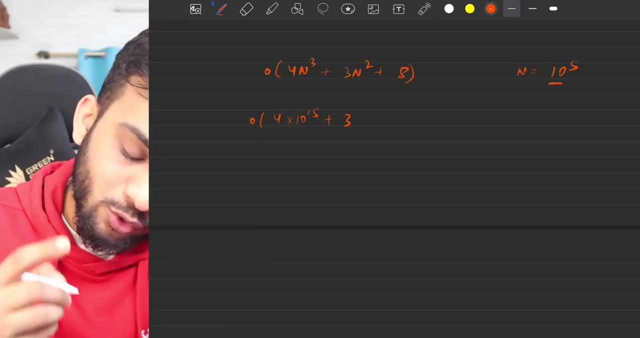 so when i say 10 to the power 5 and you put that in, what will, what will it be? 10 to the power 15, 10 to the power 5, cube 15 plus 3n square, that's 3, 10 to the power 10 plus 8. tell me a very easy. 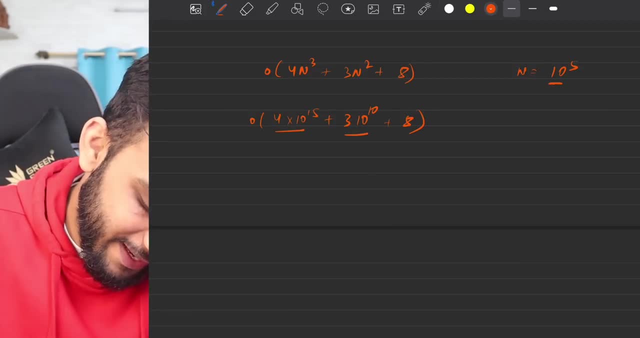 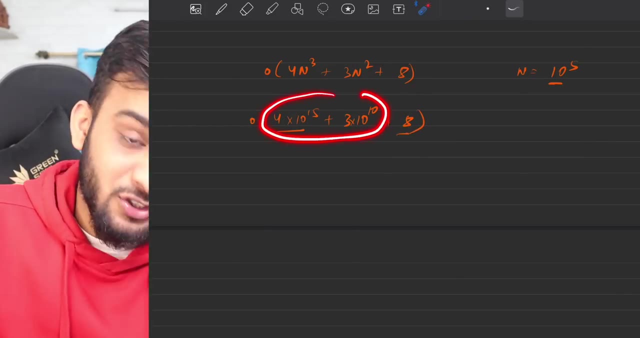 thing 10 to the power 15, plus 10 to the power 10 into plus 8. will this 8 be 10 to the power 5? will it have any significance in the operations? this is in itself such a huge number. if you add 8. 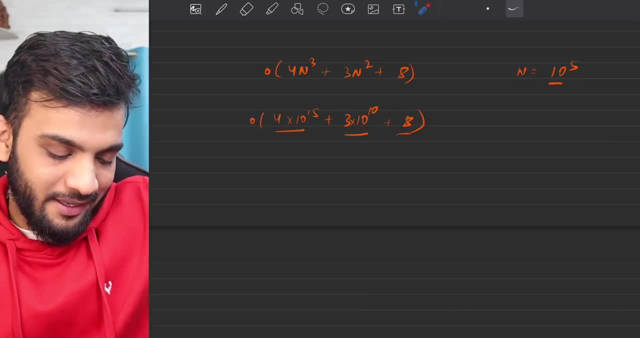 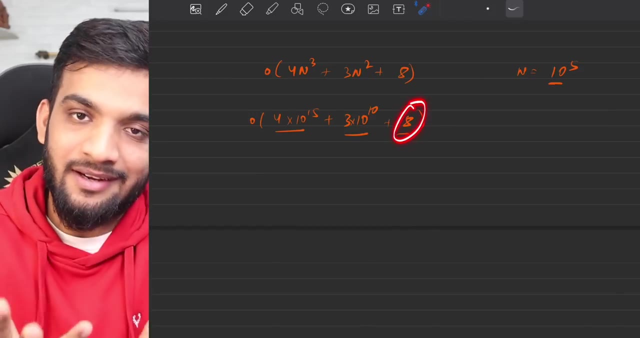 will it? will it matter to them? they're taking like billion, like whatever is 10 to the power 15? i'm not sure what it is. it's like billion, trillion, whatever, like more than that, i guess, with that a plus 8. does it have a significance? it doesn't. if you're earning 1 million and i give you one buck, that. 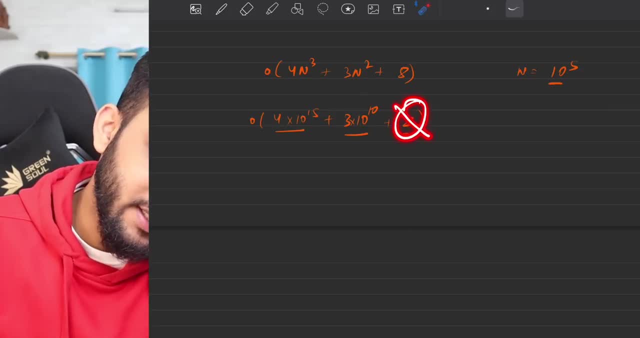 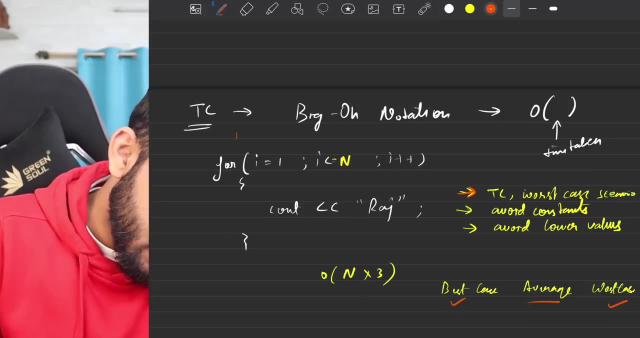 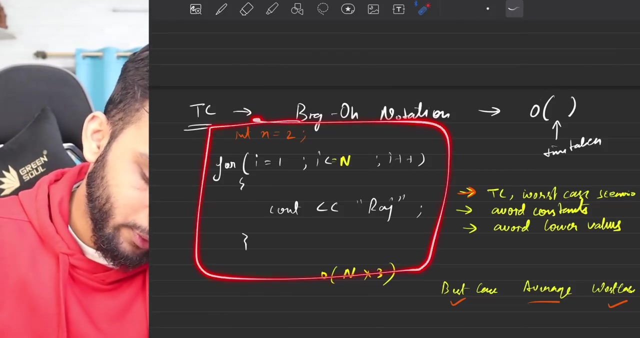 will not have any significance. that is why we do not consider constants. we do not consider constants now in terms of code. imagine, i say you something like this: int: x equal to 2. so this is the modified code, this is the modified code: x equal to 2. and then the for loop. 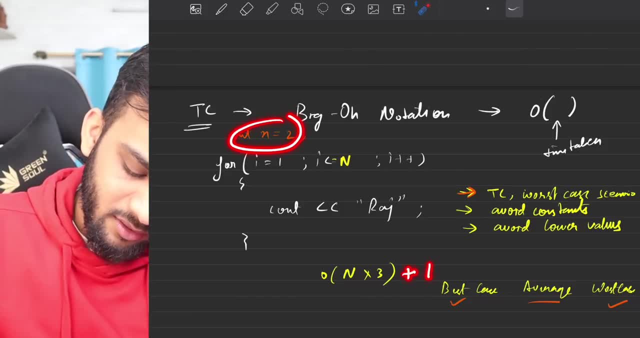 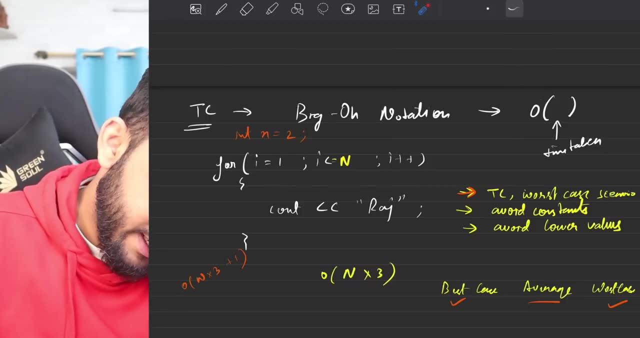 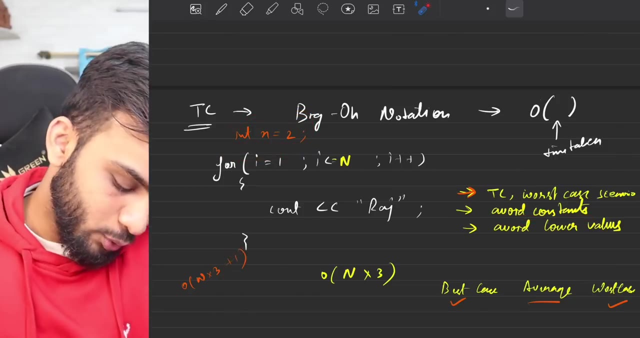 so this is one operation. it's it's something like n into 3 plus 1. the time complexity updated will be n into 3 plus 1 operation and this is the one operation. so you never, ever take this unit operation. so you will not consider this, you will say no, it will still stay as n into 3. i will avoid constants because 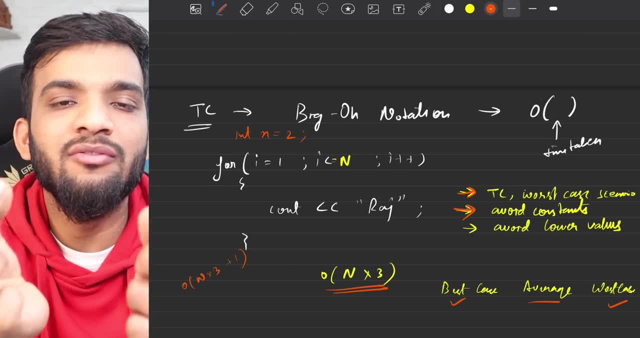 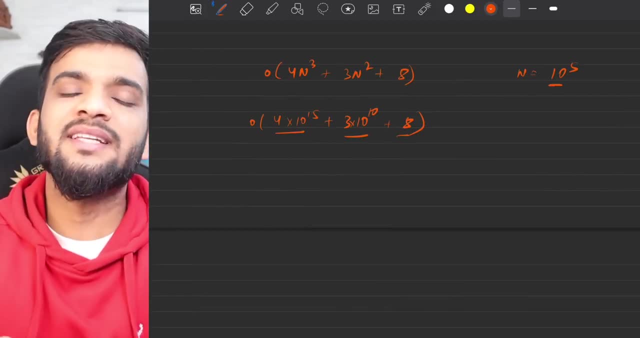 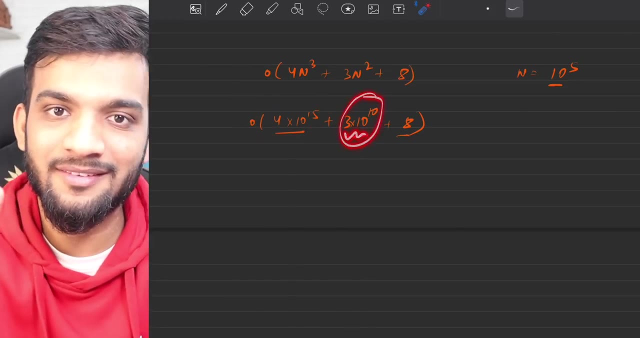 whenever the input size is very large, those constants have very less significance. got it? now let's take the next thing: avoid lower values. let's take the same example. i am saying 10 to the power of 15, 10 to the power of 15. if you add 10 to the power, 10 to it, will it have any significance? 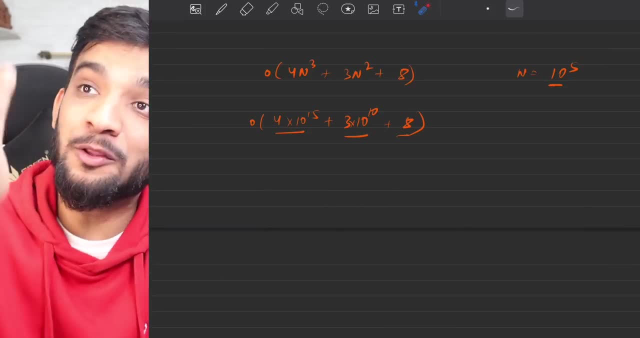 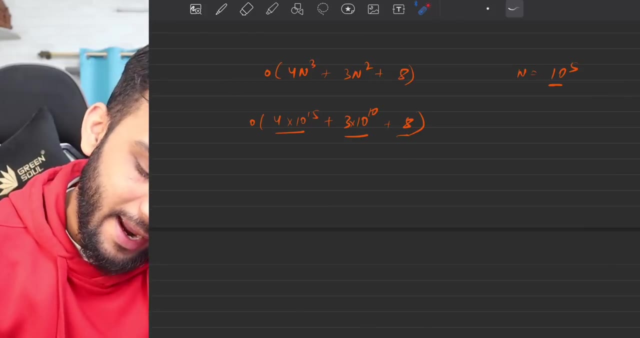 it won't. so adding 10 to the power, 10 to 10 to the power 15, 10 to the power 15, will have absolutely no significance. it is similar to saying: i will add, let's say 1 to 1000, even even lesser than that. it is similar to actually saying 1 to yeah, i'm adding 1 to this. 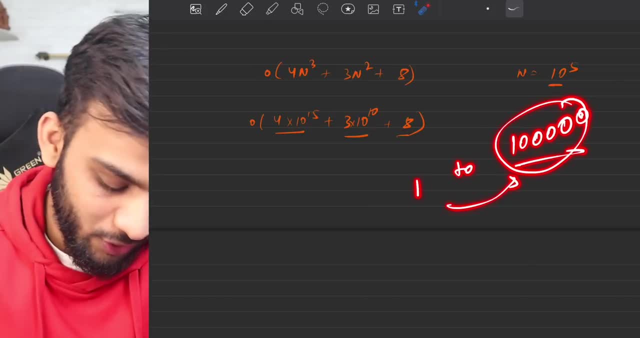 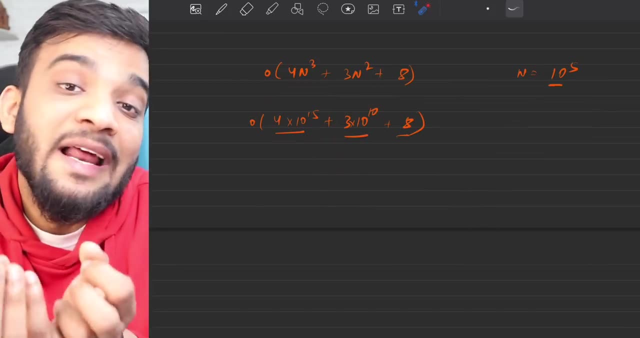 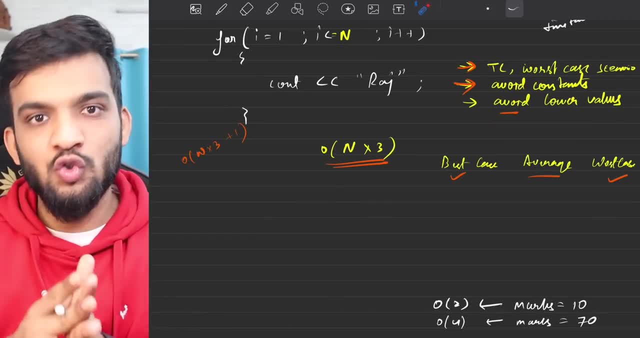 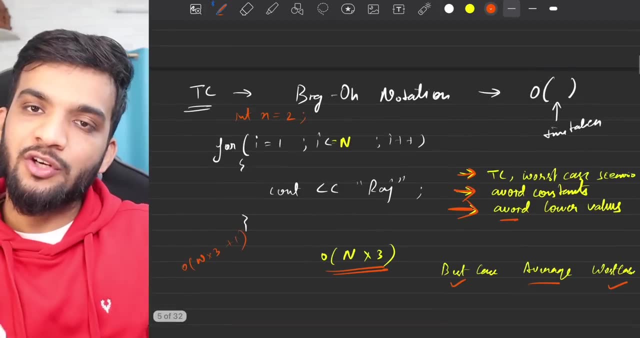 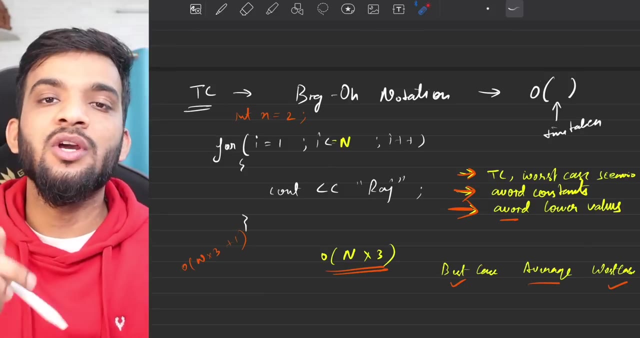 important: avoid the lower values, which does not change its significance by much. so avoid lower values, correct? so these are the three points that you will always keep in mind while computing the notation, because bigo notation is what you will be expressing, your code in interviews, always all the. 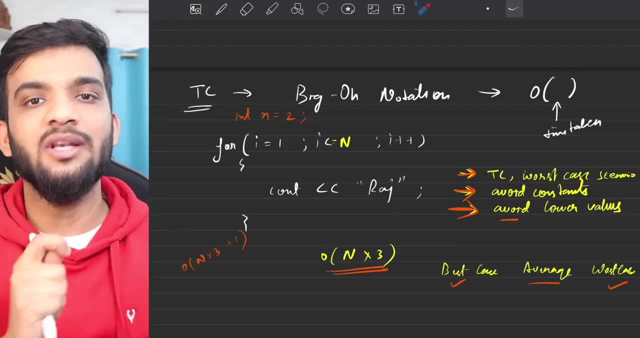 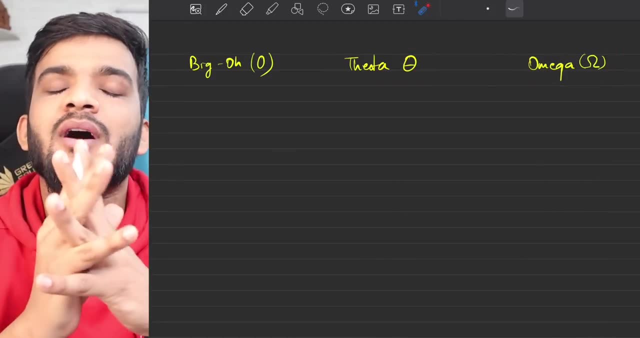 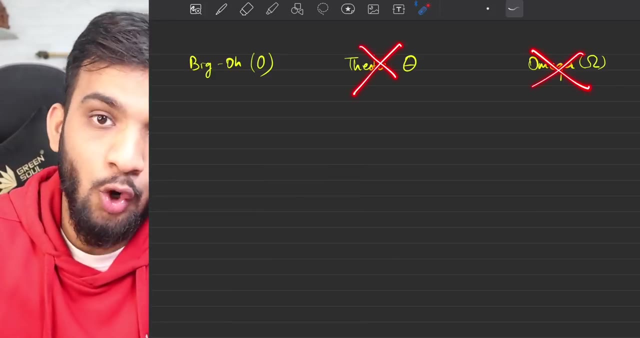 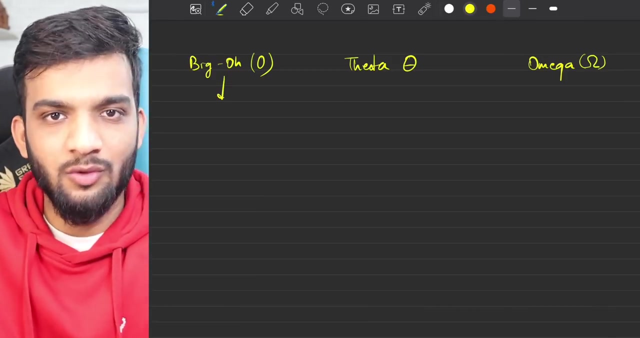 problems that i will be solving. i will be telling you about bigo notation only. apart from bigo notation, there are certain other terms like theta notation, omega notation. they will find a lot of other terms in textbooks. are they required in interviews? no, no one is going to ask you these things, no one. but just for knowledge, let me tell you: the bigo notation is always the highest complexity or the worst case complexity. remember this: worst case complexity or the highest complexity is always the highest complexity. 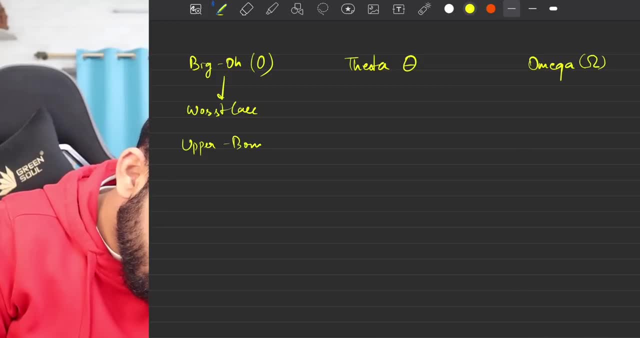 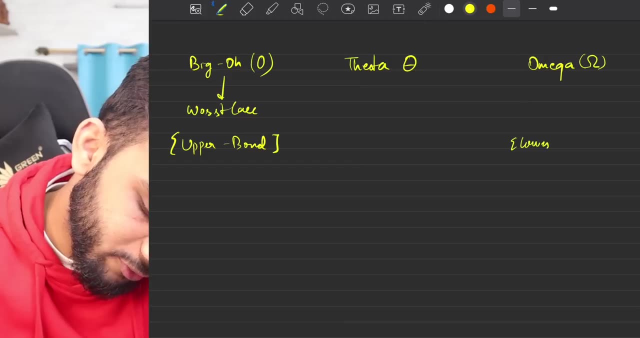 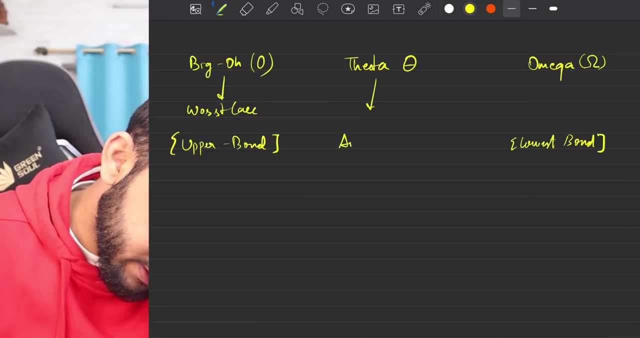 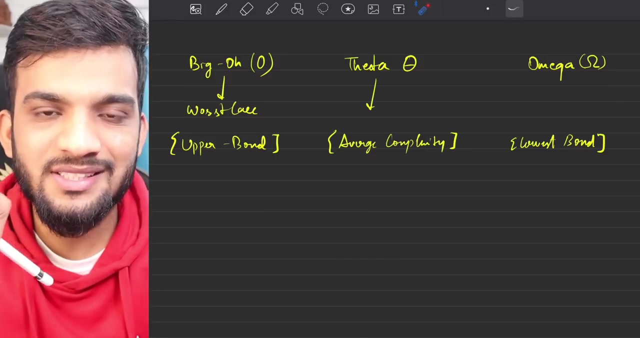 or generally known as the upper bound. complexity. it's known as the upper bound. the omega is the lower bound. as i said, the kind of the best case is the lower bound or the lowest bound or whatever you can. and this is nothing but the average complexity. just a quick disclaimer. there are 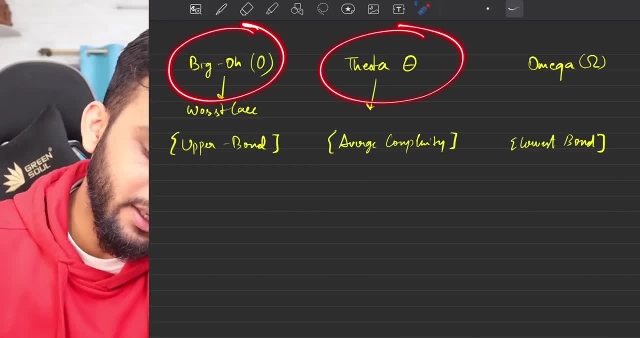 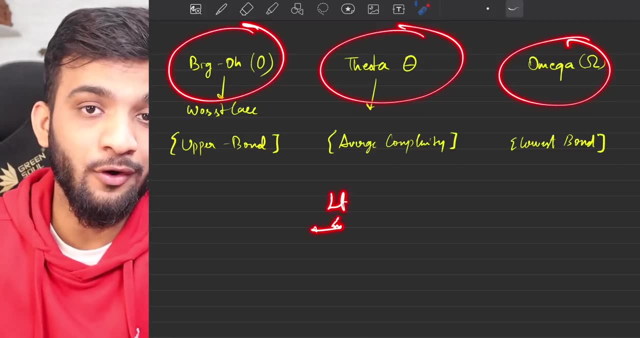 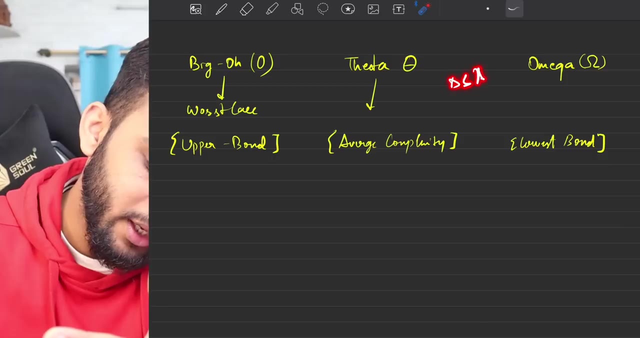 a lot of theoretical stuffs revolving around bigo, theta, omega, a lot of limit derivations. but i'm not teaching you theory stuff. i'm not teaching you for your semester examinations. i am teaching you for interviews. i'm preparing you for the dsa coding rounds and they will not be. 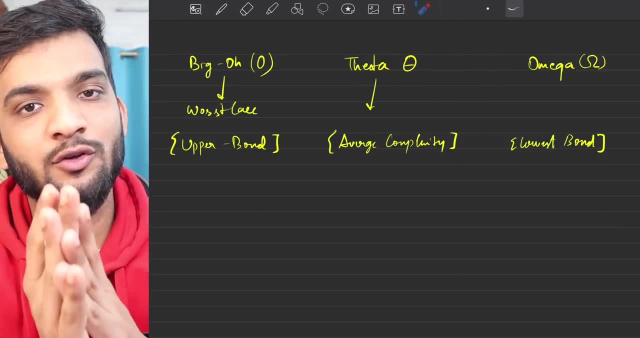 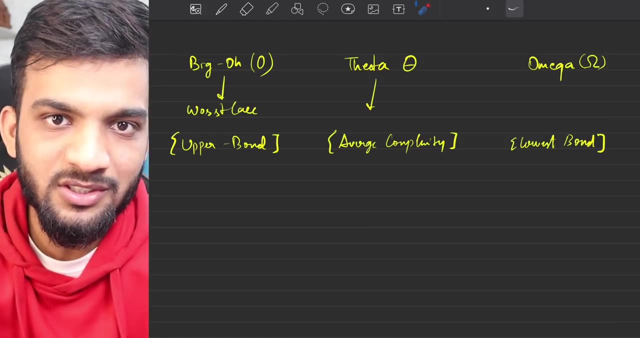 asking it over there. they'll be asking you programming logic. you'll have to solve problems. they won't be asking you tell the formula for bigo notation in limit terms. no one is going to ask. might be asked in semesters for that. you'll find different teachers on youtube. if you're learning from me, you're. 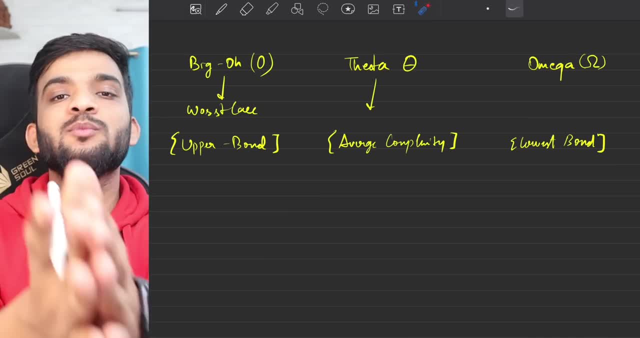 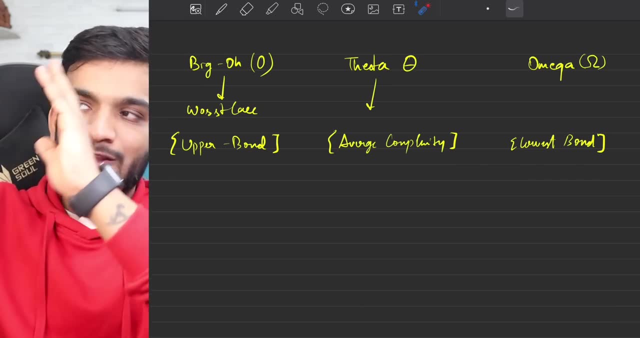 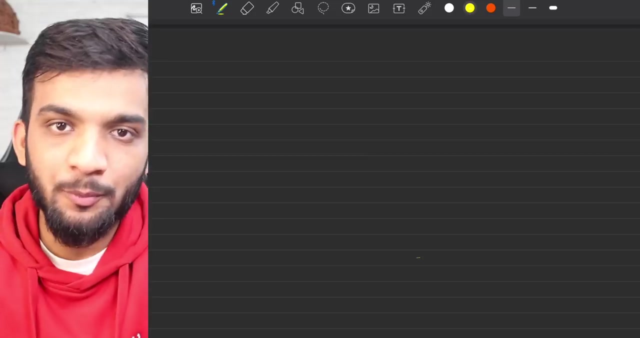 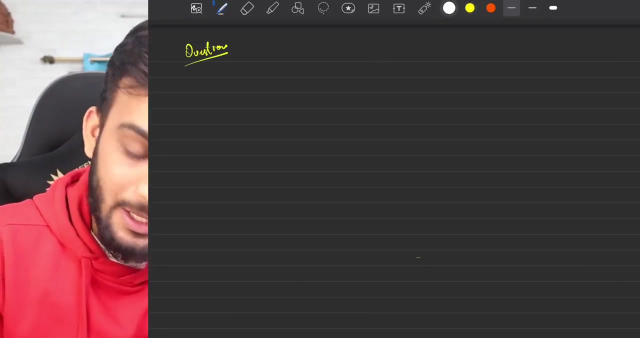 learning for interviews, for coding rounds, for problem solving abilities, not for your semester exam. so please do not comment that you did not teach the mathematical derivation, because that is something which is not required while problem solving, right? so you know how to compute bigo. now let's do one thing. let's quickly solve some questions. okay, so the first snippet of the 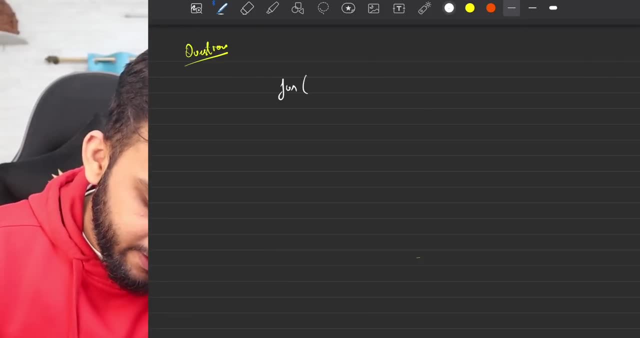 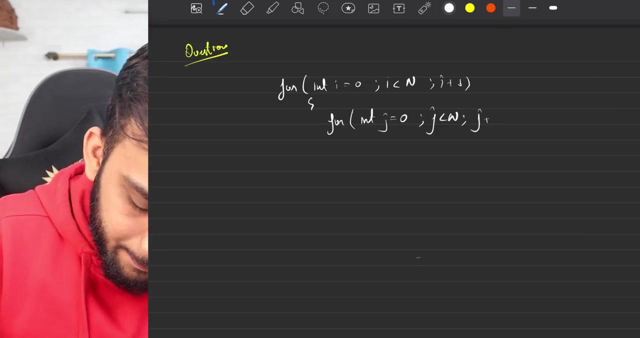 code for which you have to find the time, complexity. imagine inside your main you have something like int i- equal to zero, i less than n i plus plus. and for int j, equal to zero, j less than n j plus plus. and imagine it has a block of code like something, a single line of code and this is your entire. 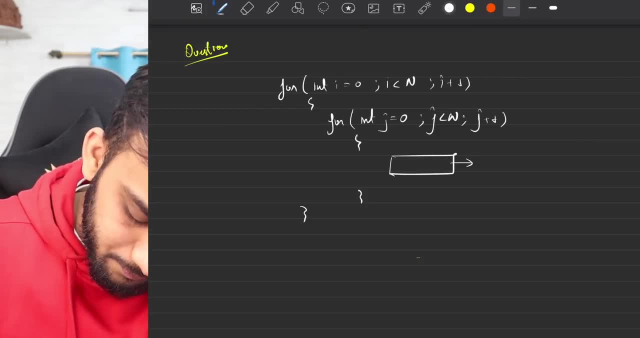 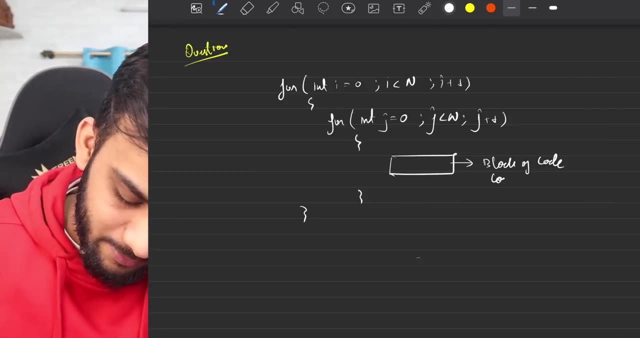 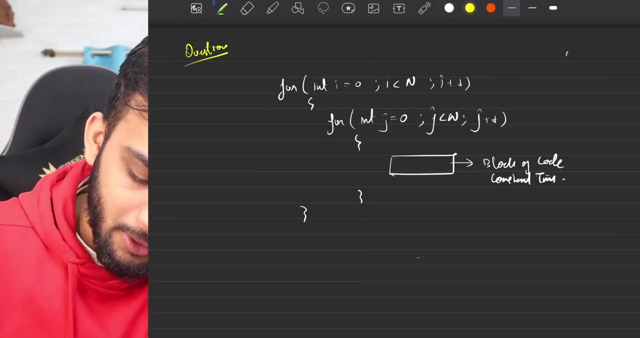 snippet of the code. okay, this is your entire timeline of that particular type of block in which my line is and i have a billion blocks of block in which my line is and i have a billion block of code. you can consider this to be taking very constant time, constant time. so this can be avoided, tell. 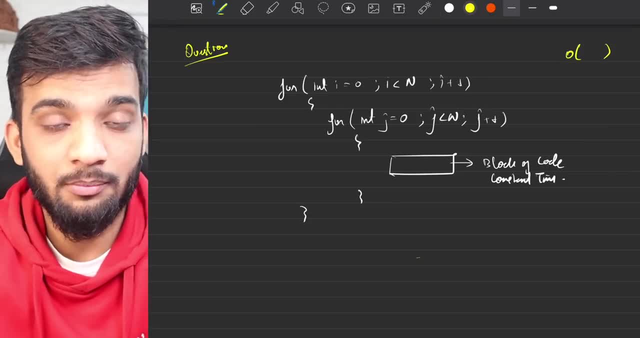 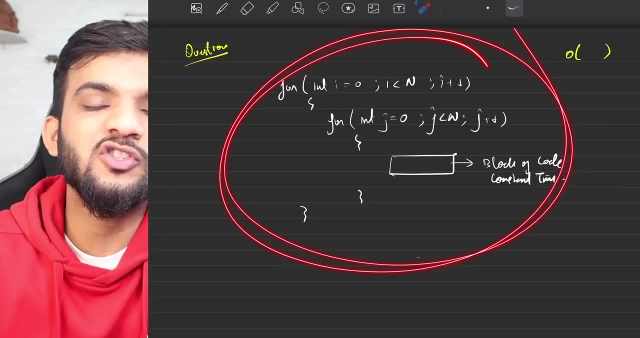 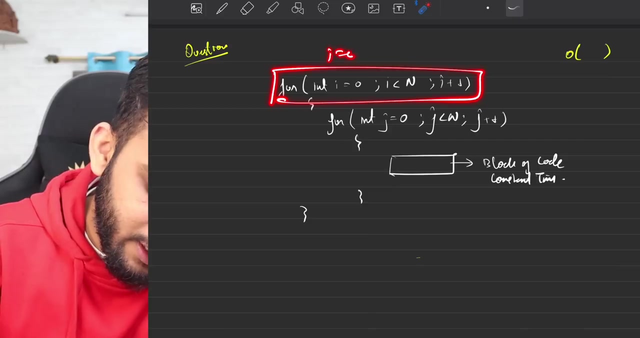 me the time complexity. you know time complexity will be computed in terms of bigo notation. tell me the time complexity of this particular code. pause the video and maybe think about it and then see if you are correct or not. so how do you analyze the? is the code working? so, if you see, the outer loop is starting from i, equal to zero, and going till n. 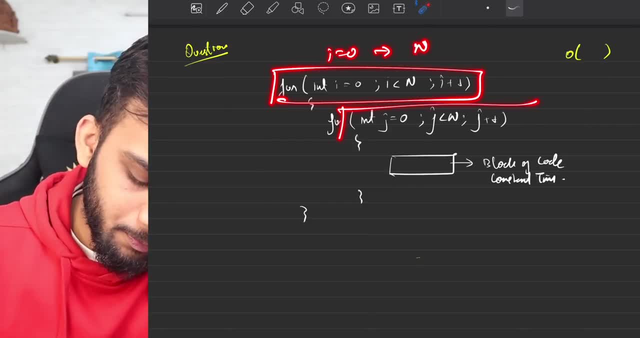 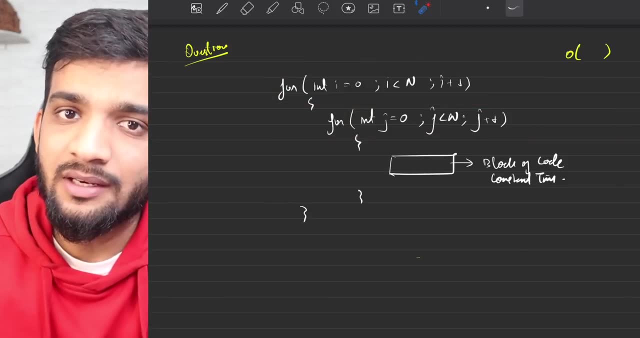 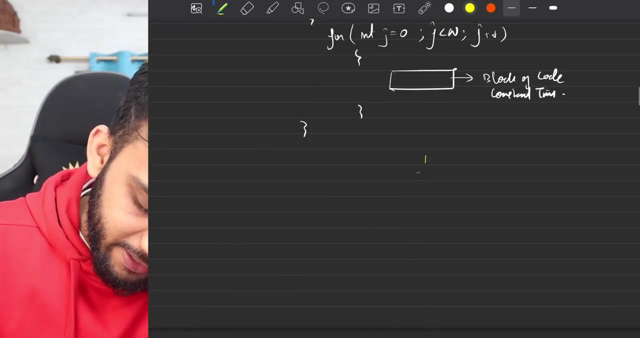 that's definitely running for n types, and the inner loop is going from j, equal to zero, till n. this is also running for n types. now, if you're a beginner, you might find it a bit difficult. so what you will do is you will say at i, equal to zero. what is happening, let's see whenever i is zero. 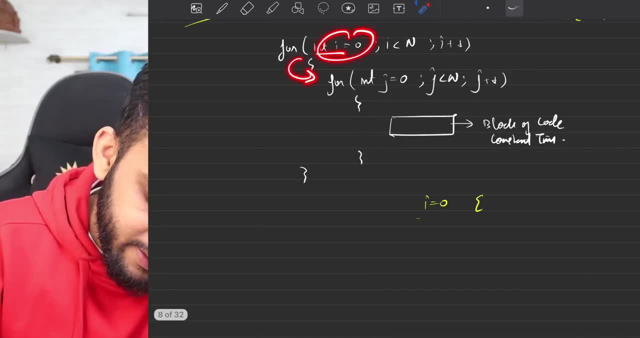 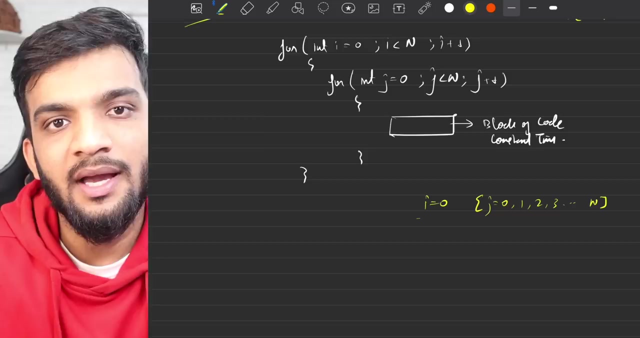 what is happening? whenever i is zero, it goes inside and j starts its value from zero and goes till n and this completes n iterations. can i say: when i is uh, zero, j goes from one, zero, one, two, three, dot, dot till n. can i say? and then again, when the i is, value increases to one. can i say? 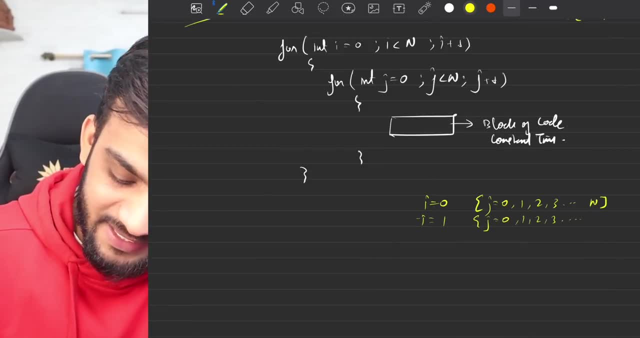 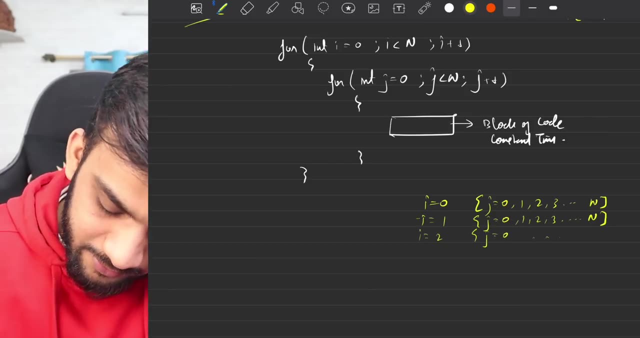 j again goes from zero, one, two, three. because it's inside it. it's reiterating: again from zero. can i say: if i is two, again it again goes from zero till n. can i say: till i is n minus one. why n minus one? because it is. 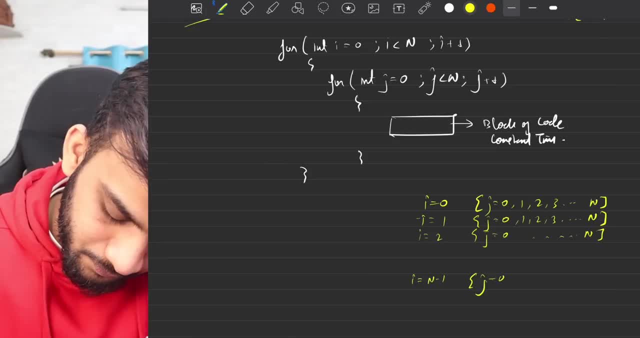 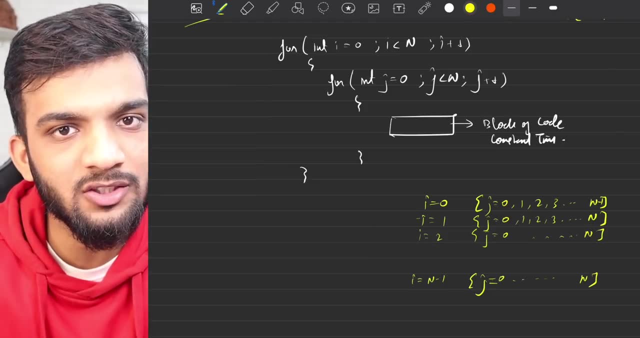 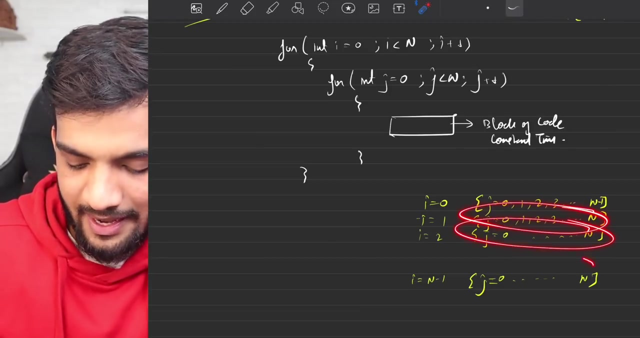 lesser than n. can i say it again goes from zero till n, or rather than n minus one, to be very accurate. can i say this? so what is happening? every time? it is running for n, n, n, n. every time it is running for n and n. so can i say it's running for n. 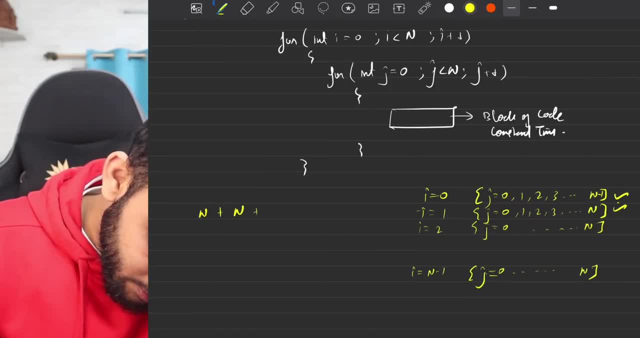 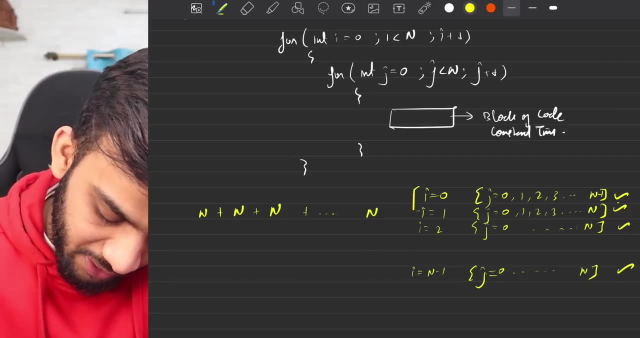 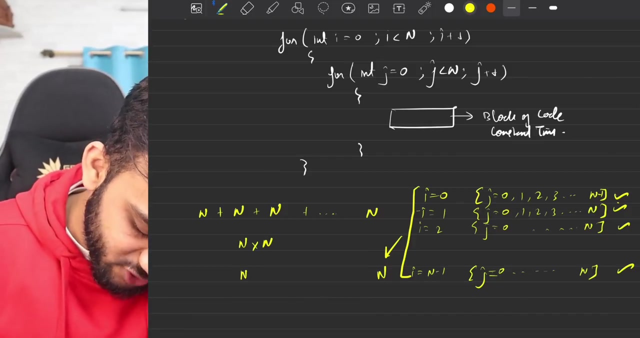 times first, then for another n times second time, then for another n times second, and then dot, dot, dot, dot till n times. how many times is it running? can i say it's running for exactly n times. so can i say this is nothing but n into n? yes, thereby n square is the number of iterations. 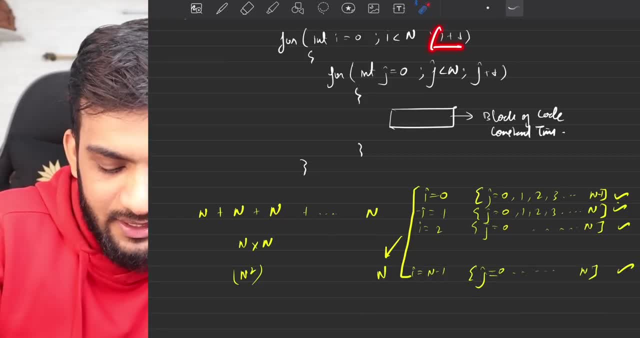 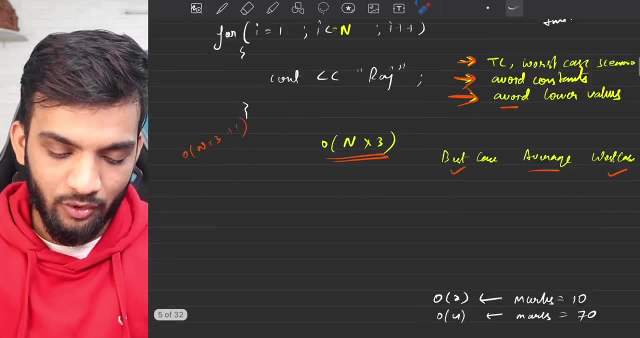 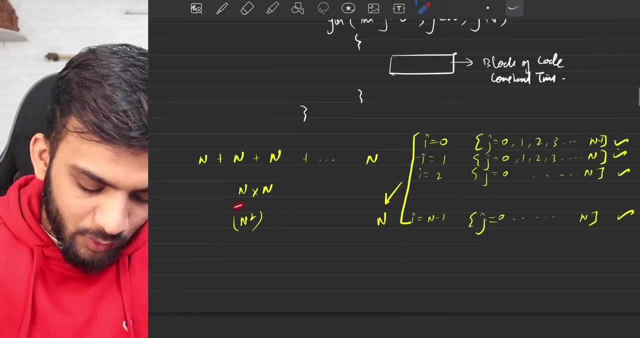 it is taking. yes, there are other things as well, like increase comparison, but we usually do not consider which rule. avoid lower values, if you remember, because three into something won't matter that much. yes, you can avoid it. what i can say is: it's running for n square. yeah, if you want to consider all these constant. 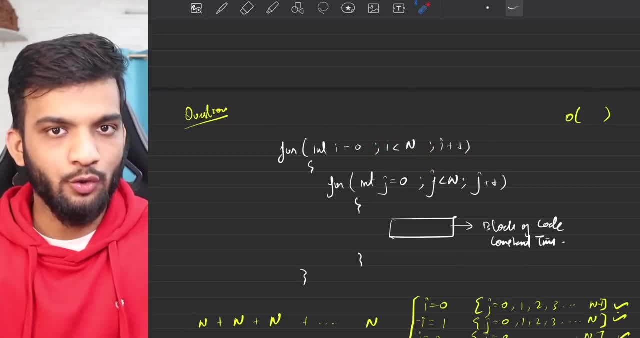 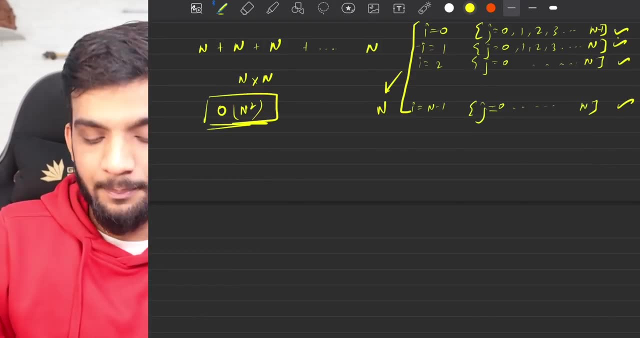 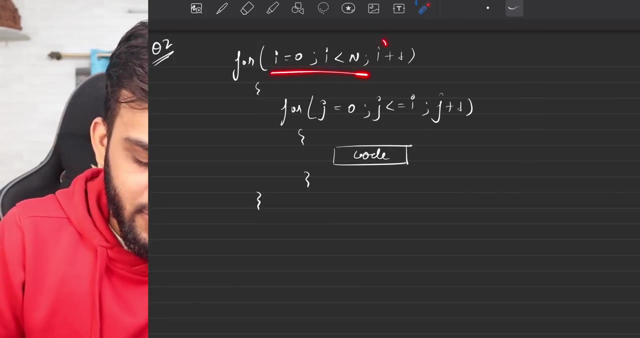 operations. you can do it that is your wish. i usually do not do it, so b go of n square is: what is the time complexity of this particular? let's take the next example and try to compute the time complexity of this one. so it's like the first loop is: 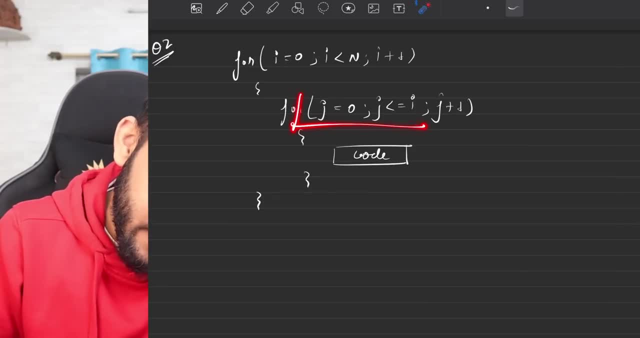 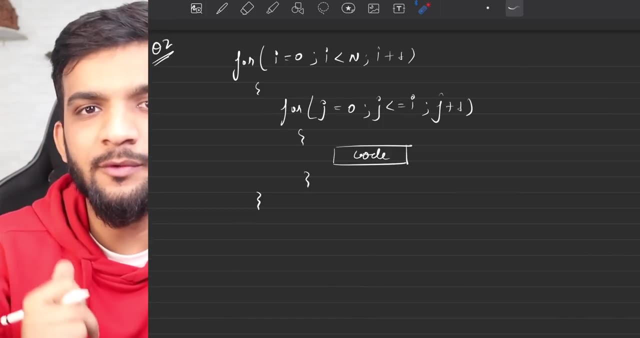 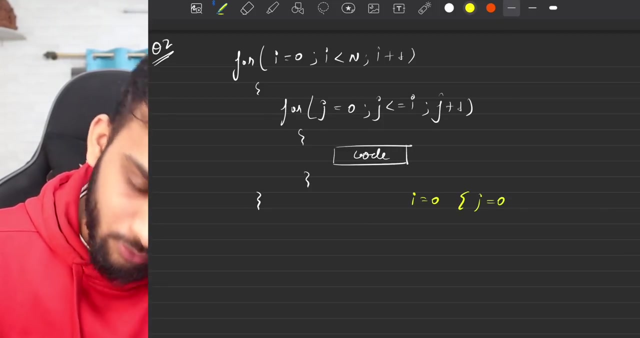 definitely running for n and the second loop is running from zero to i. so let's analyze slowly and probably we'll get the time complexity. so can i say, if i equal to zero, j is nothing but from zero is only running for zero. can i say this? because when i is zero, j is running for zero j. 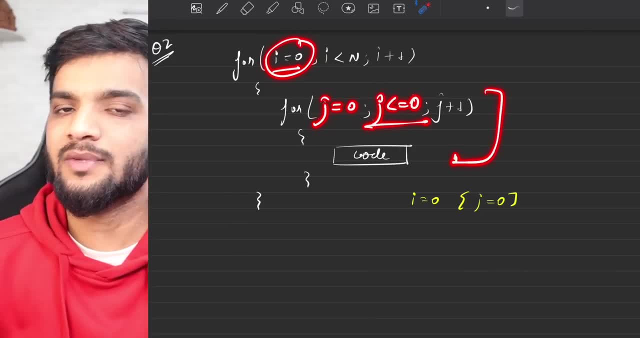 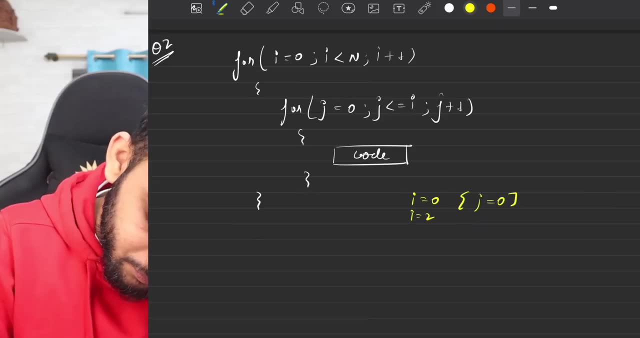 less than equal to zero, it will run for just one time. well, when i becomes two, what happens? j now runs for zero. sorry, when i becomes one, rather, when i becomes one, what happens? j now runs for zero and one. can i say why? because i is one. it's like zero lesser than one, correct? 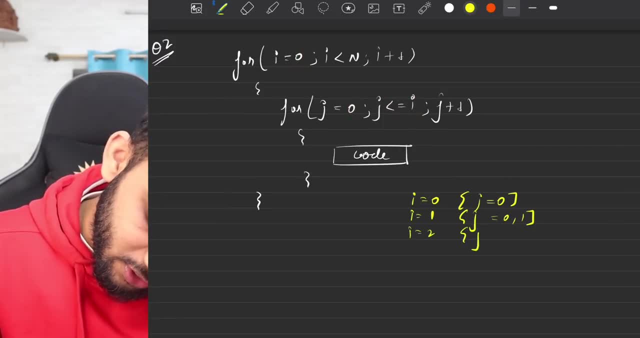 nice. can i say, if i is equal to two, what happens? j now runs for zero one two. so when i at the end becomes n minus one, what will happen? j will be zero one, two. dot, dot dot n minus one. can i say this is how many operations i will get when i becomes one, and when i becomes two i will get. 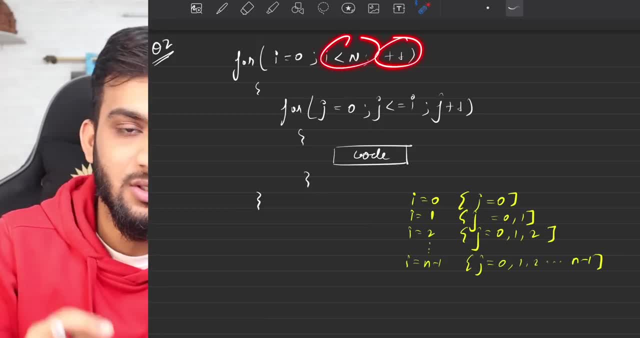 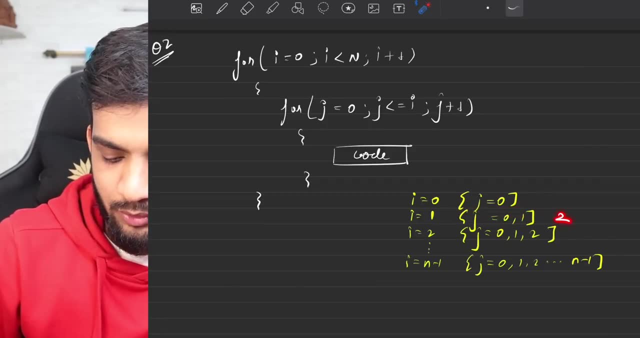 n minus one. so this is how many operations it is taking. again, i'm ignoring all these constant operations. i'm taking the overall iterations now. the first time it's one iteration, next time it's two, next time it's three, four until n. so can i say the number of iterations? the first time it is? 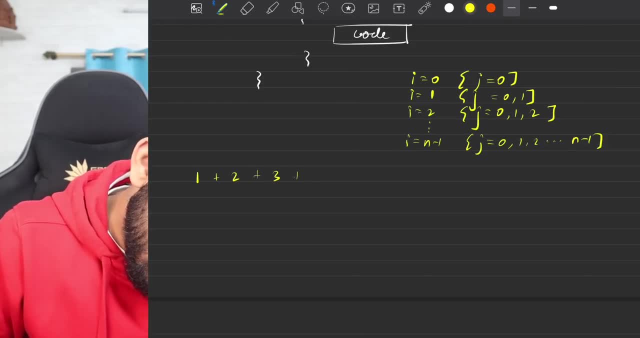 one, the next time it is two, the next time it is three, the next time it is four, so on till n. can i say, and do you remember the formula for this particular thing, some of the first n natural numbers? simple math: n into n plus 1, whole divided by 2. 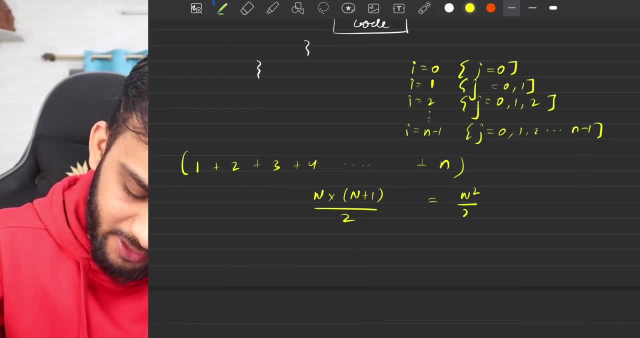 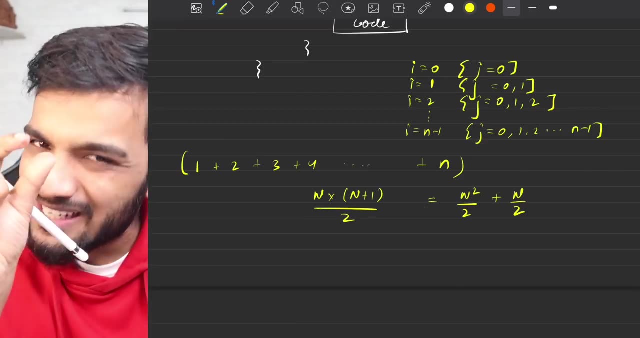 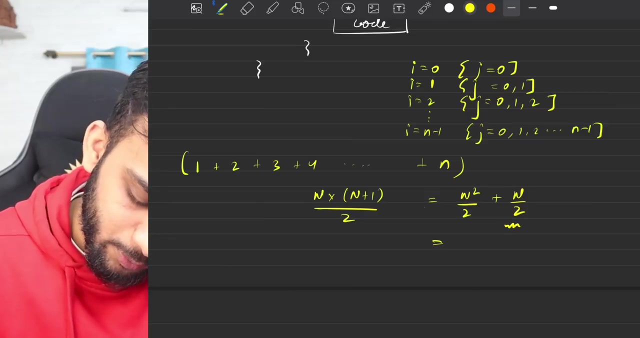 which is nothing but n square by 2 plus can I say n by 2? thereby, this is the exact time complexity, but we can avoid, if you remember the rules, constant to be like the smaller values to be avoided. so it will be like n square. 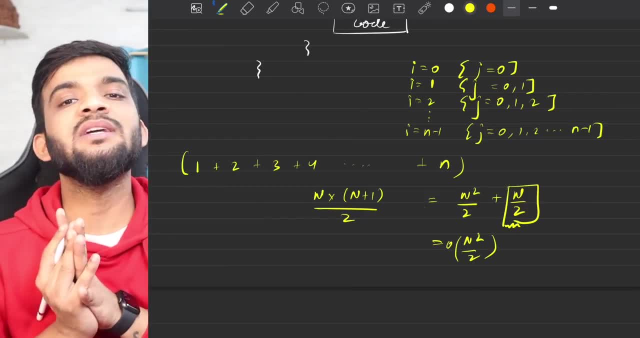 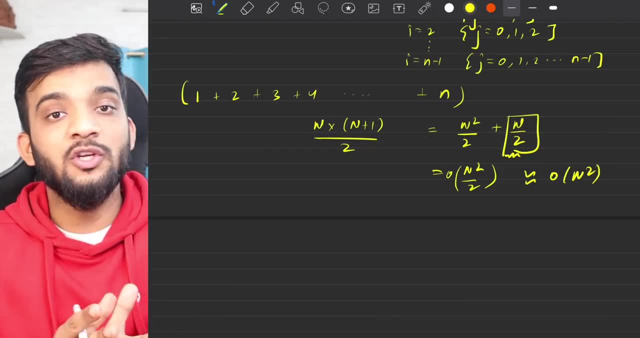 by 2, so this is the time complexity. again, if you try to remove the constants like 1 by half, you can say the time complexity is near about, we go of n square. but if someone does ask you the exact time complexity, this is the exact. 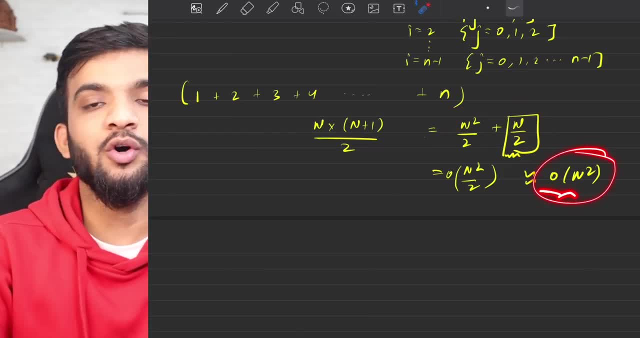 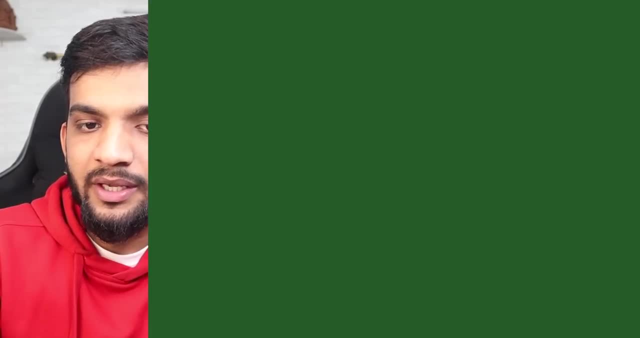 time complexity, but according to the rules, this is what it boils down to. so these were the basics of time complexity. okay, now. next, I'll be doing all these patterns in the next lecture, where I'll be writing all the nested for loops. 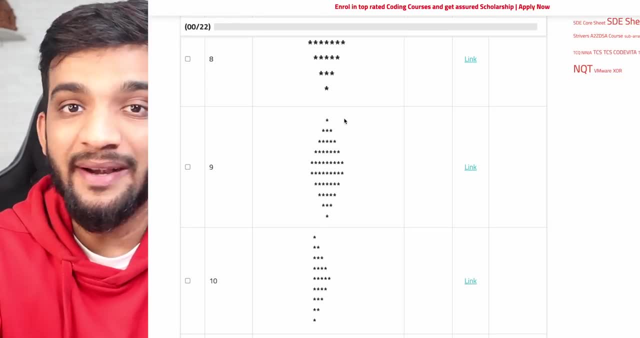 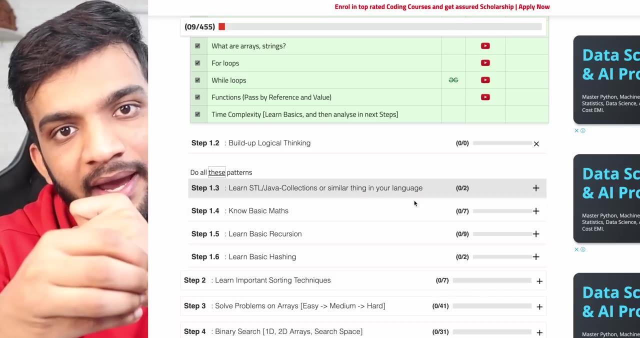 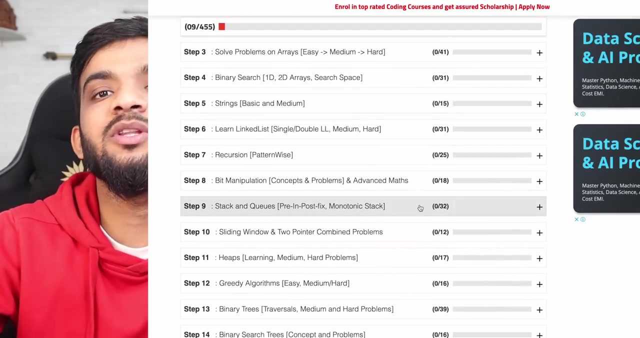 and there you can analyze time complexity in a much better way. but eventually, all the time complexity terms like log n n, log n n square n, cube n, square log n, all of these things you will see as I proceed with the playlist. I do not want to rush you in. 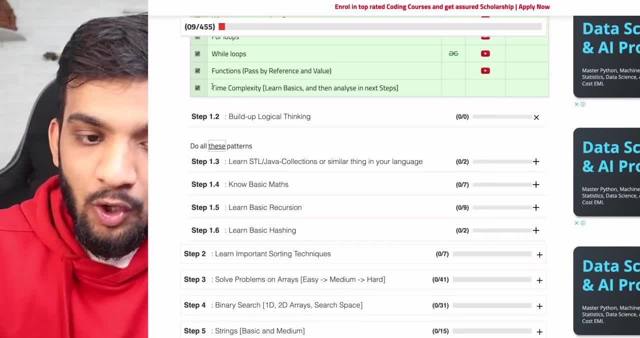 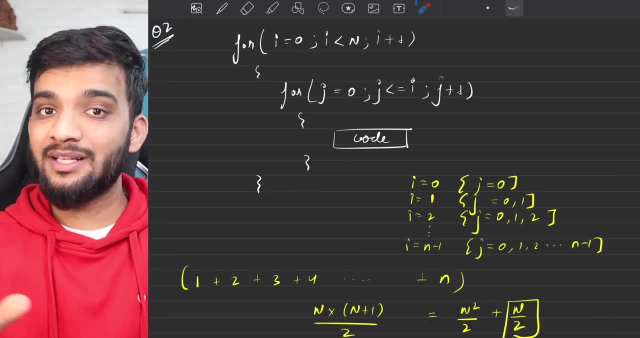 I just want you to get an overview of what is time complexity, how to think on it, how to compute, how to avoid terms. these things should be crystal clear to you. so I'm assuming the time complexity stuff is crystal clear to you. so I'll now be moving to something like space complexity. 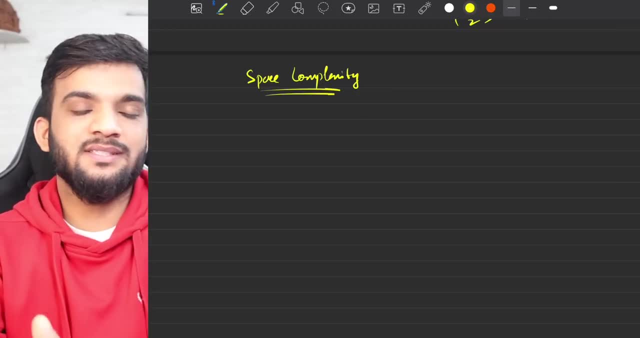 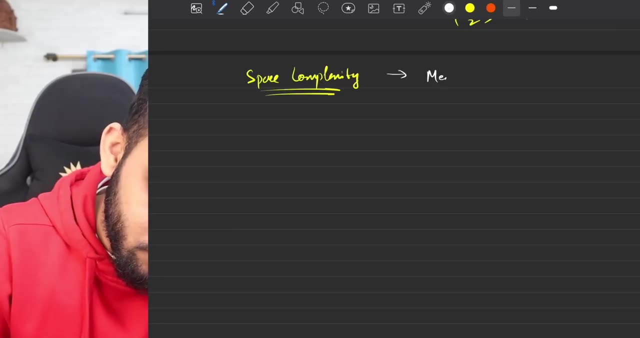 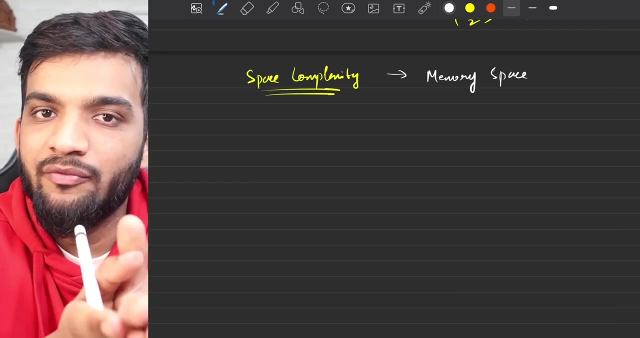 again, what is space complexity? it's the memory space that your program takes. it's the memory space that your program takes in a very, very naive term. when I talk about memory space, again, it will vary from machine to machine, so you cannot be dependent on. 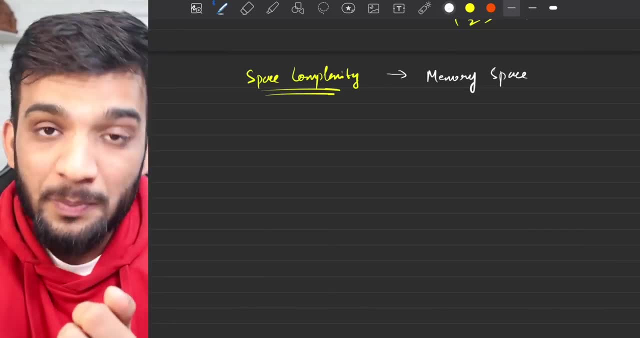 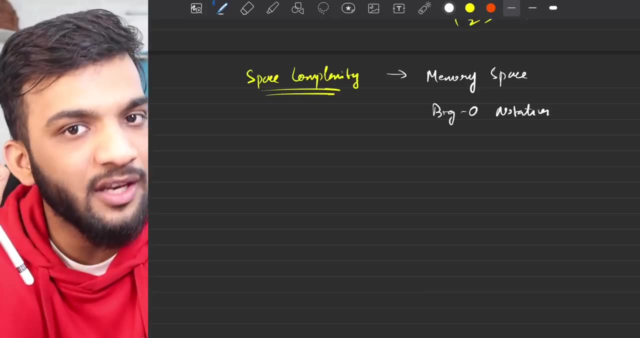 the machine. and that is why, again, in order to compute space complexity, we will be using the Beagle notation again. so Beagle notation is kind of very, very important in all the interviews: Beagle in terms of time, Beagle in terms of 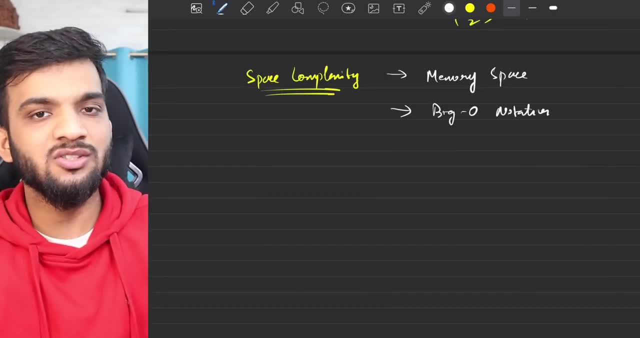 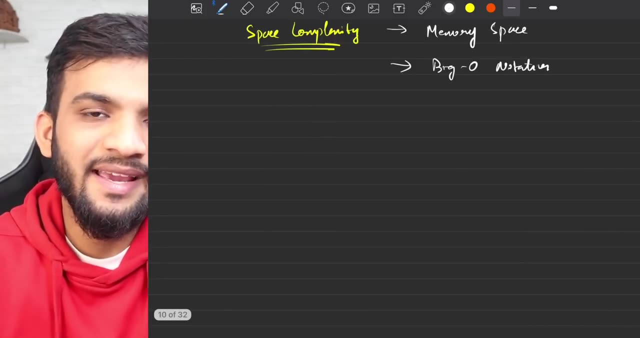 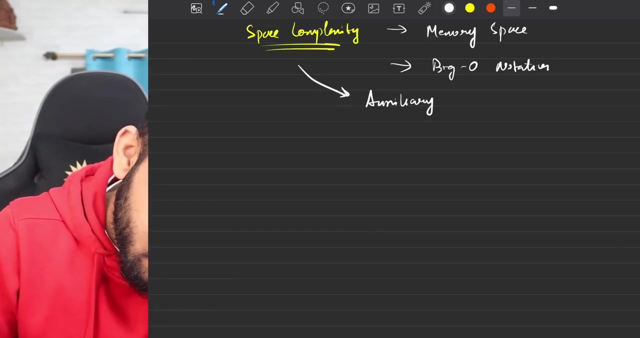 the space. so we'll again be using Beagle notation, and you know the reasons why: not in terms of Kb, Mb, Gb, etc. so what is exactly the definition of space complexity? It is nothing but auxiliary space plus input space. 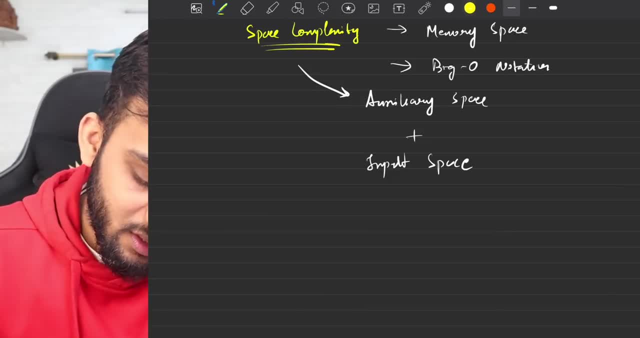 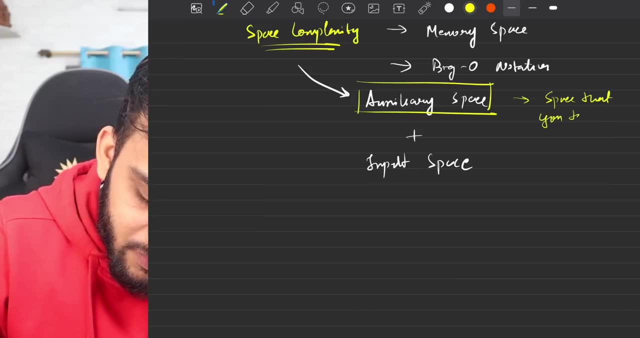 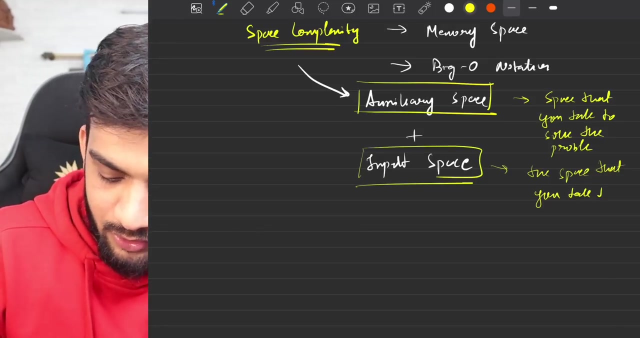 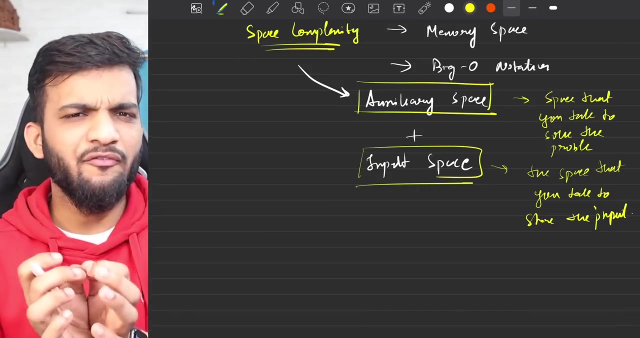 what is auxiliary space? The space that you take to solve the problem, the space that you take to solve the problem, input space, the space that you take to store the problem, space that you take to store the input, rather not the problem. so let's give a very, very small example. 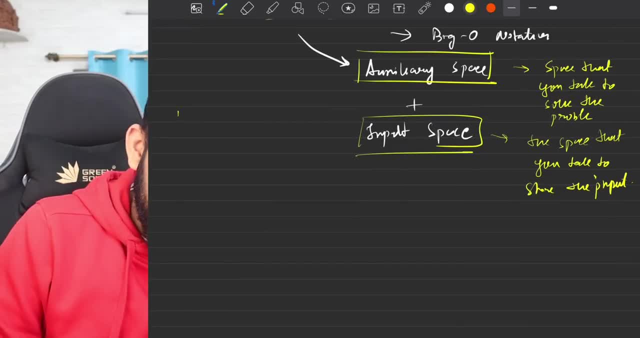 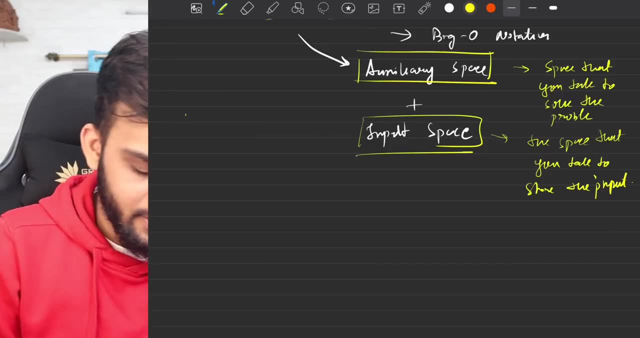 in order to explain what is auxiliary space and what is input space. So I will write a very, very small thing. imagine I am taking an input of A and B In java. you know how to take it and c++ you know. so I am assuming I'm taking an input of A. 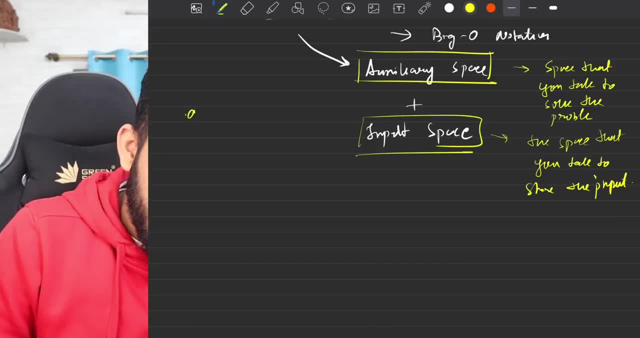 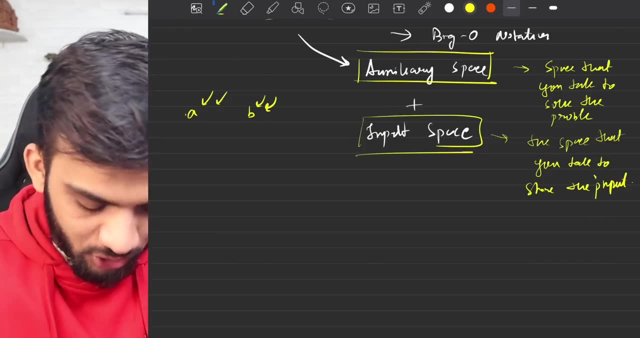 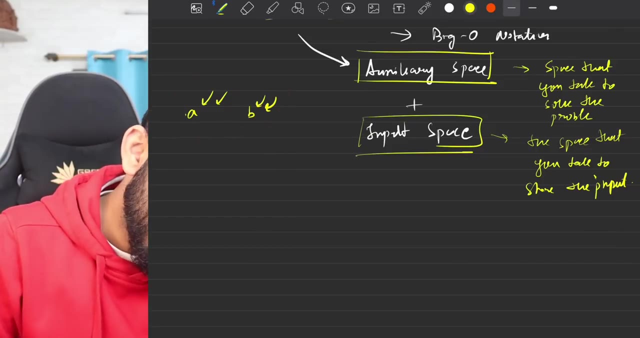 of a. uh, so i'm not writing any syntax, because then it will be c++ or java specific. i just want you to learn pseudocode and the logic. so in imagine i give an input to variable a. imagine i give an input to variable b and i am saying c equal to a plus b. now i am saying c equal to a. 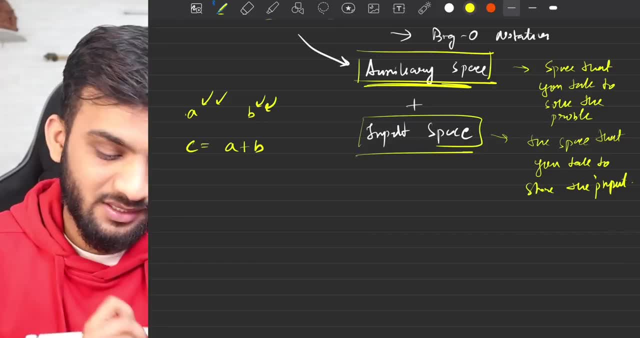 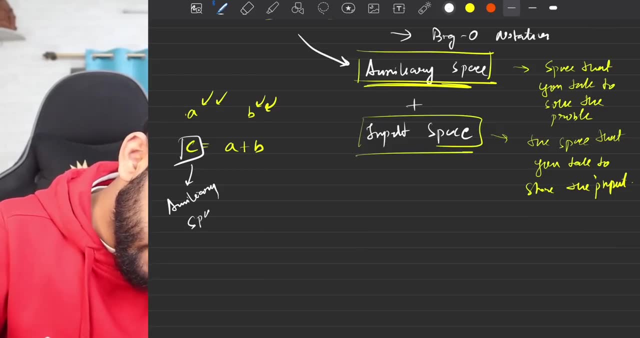 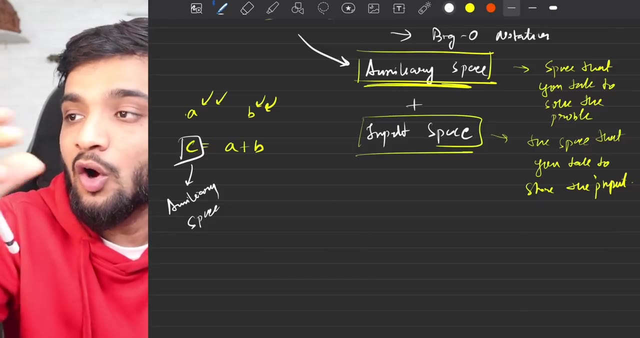 plus b. so the auxiliary space that you're using is an extra c variable. this is the auxiliary space. why? because you're using a c variable in order to solve the problem. you cannot use. that is okay. i'm saying, if you use any extra variable or extra space to solve the problem, that is what you refer. 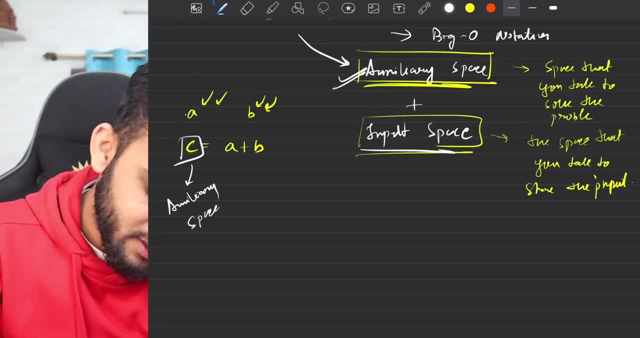 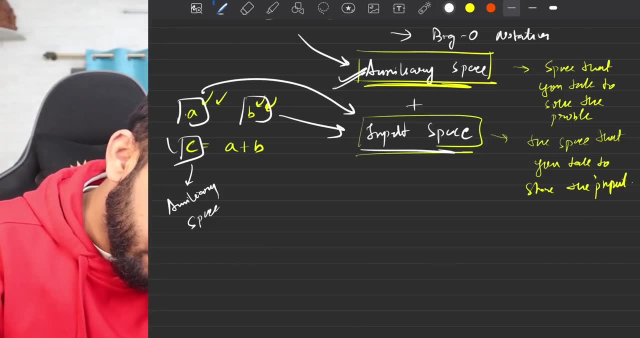 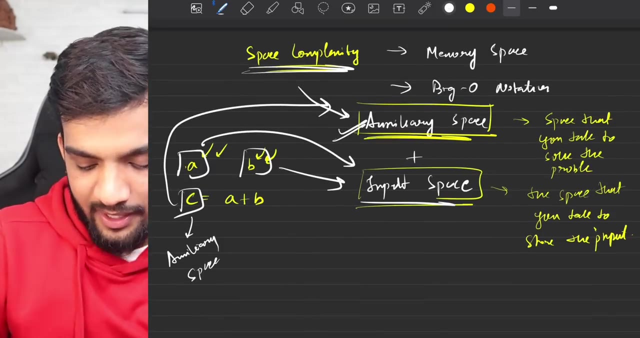 as auxiliary space. what about the input space? this is one and this is one, so both of these can be referred as input space, whereas this can be referred as auxiliary space and combined. i can say this is the space complexity, or i can say we go of three over here because you're using three. 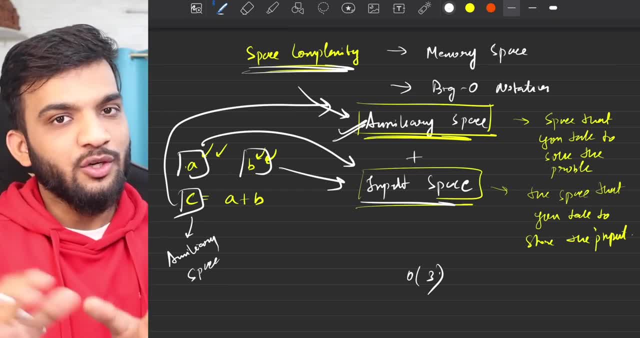 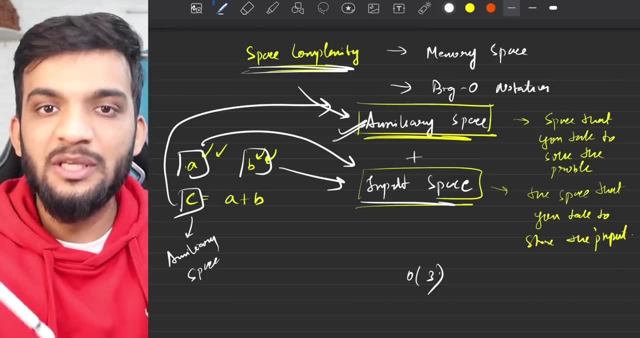 different variables, you can convert them into bytes. if you're taking integer, you can convert them into bytes. i am not concerned about this. in an interview you will have to say it in terms of we go of something, not in terms of bytes, kb, mb. so, for an example, 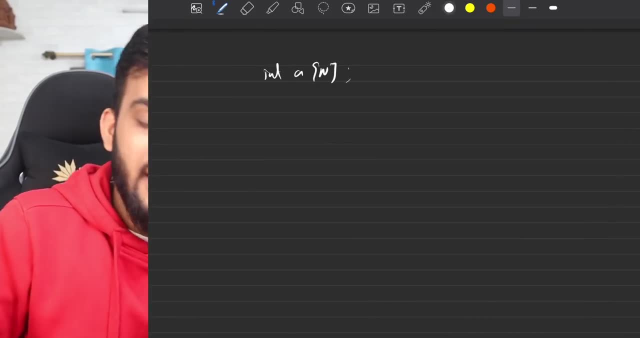 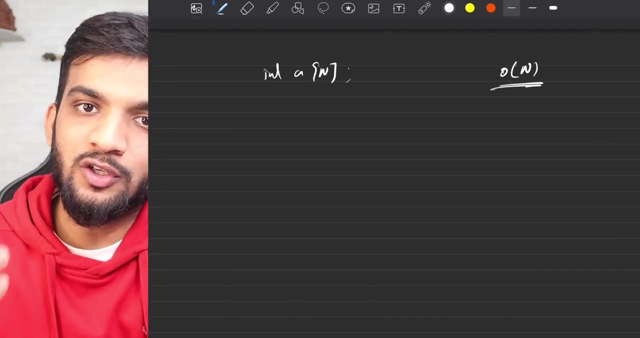 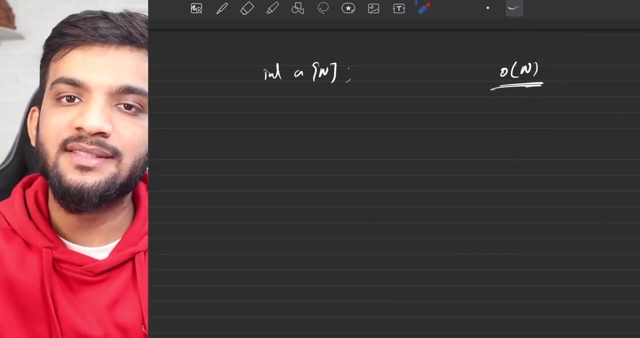 If I define an array of size n, it means I'm consuming bigo of n size or n space complexity. So in an interview, if you're solving a problem which uses an array of size n, you say bigo of n is the space complexity that I'm using. 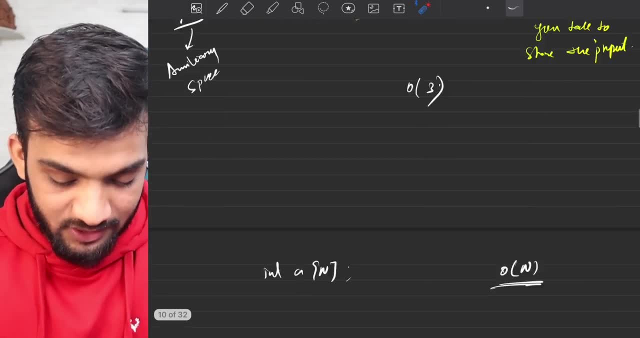 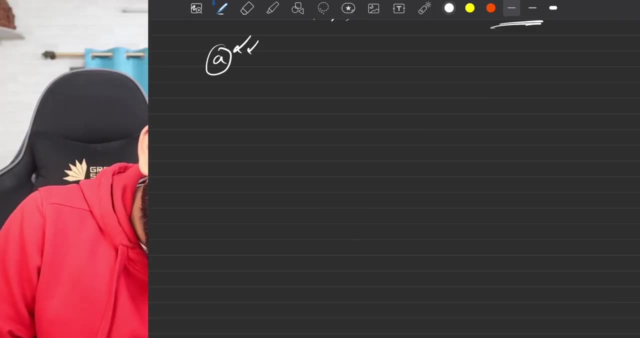 As simple as that. Now, a thing that I want to highlight over here is, if you're doing space complexity- a lot of times it will happen is: imagine you're given an input to a, imagine you're given an input to b and the task is to sum, add both the numbers. 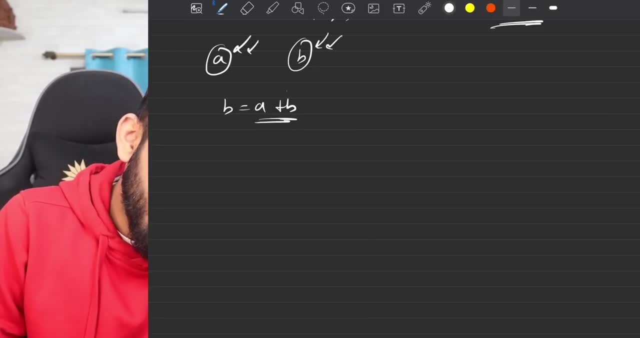 A lot of people say I'll do this. b equal to a plus b, So the summation of a plus b will be stored in b and I'll not be using the third variable. It is okay to do. It is okay. 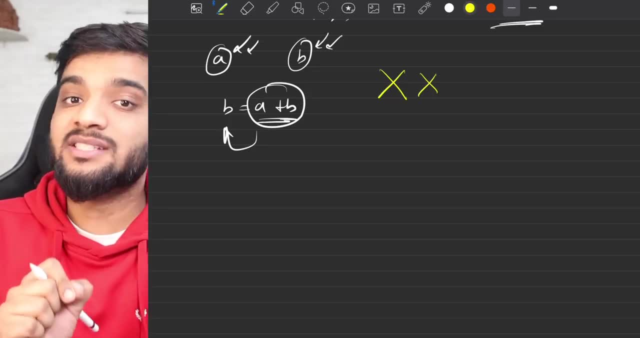 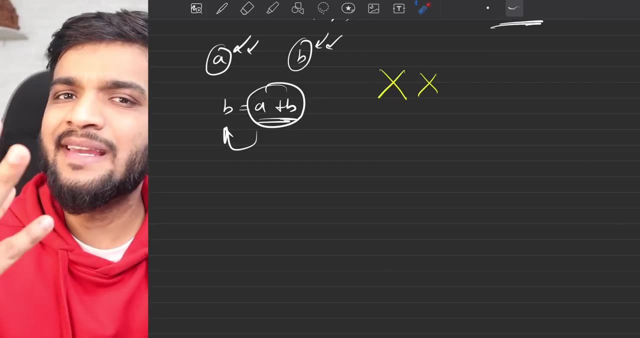 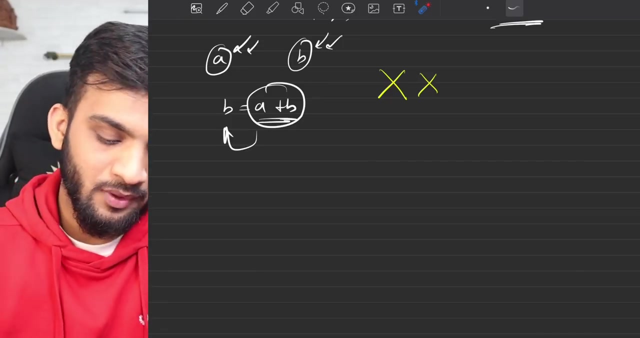 But this is something you should avoid. It takes less space, but in an interview the interviewer will say: this method is not done. Why is it not done? Just think in perspective of software engineering. Imagine you are writing a code for a big MNC and they're giving you some data. 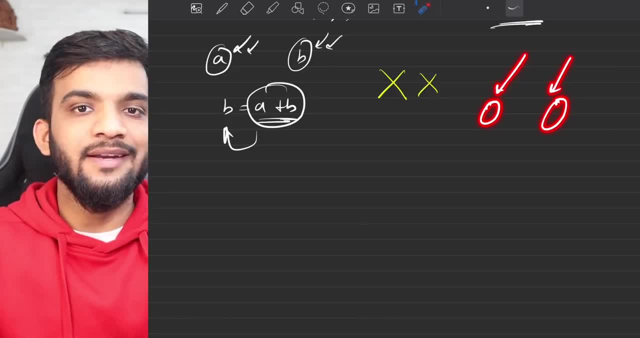 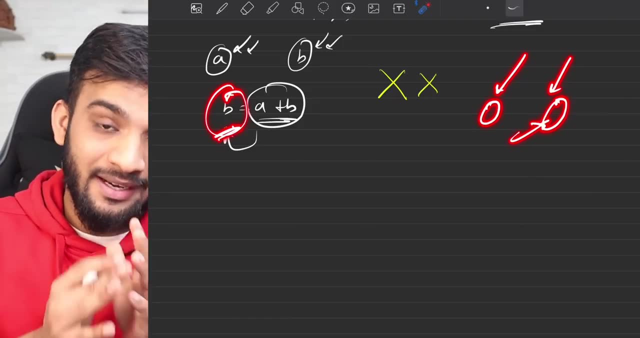 They've given you some set of data and they want you to do something on that data. And you're like, you manipulate the data Over here. you change the data, You change b. This is why never, ever, do anything on the input. 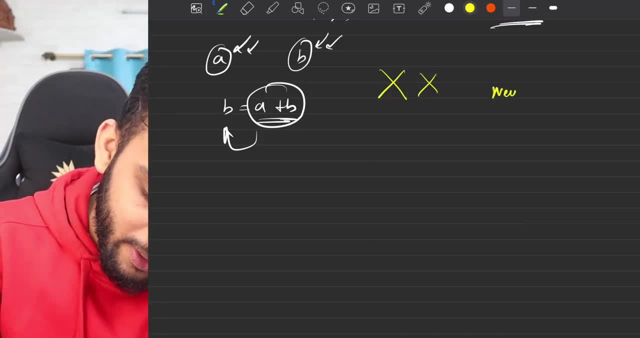 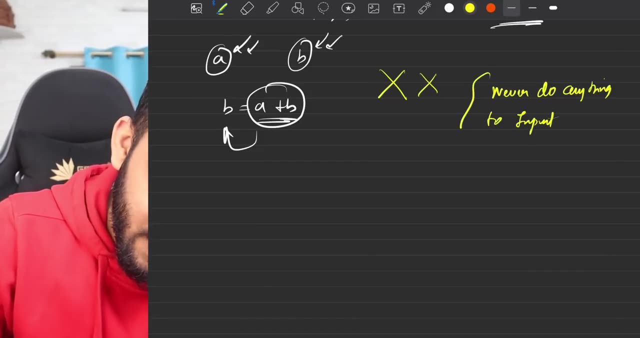 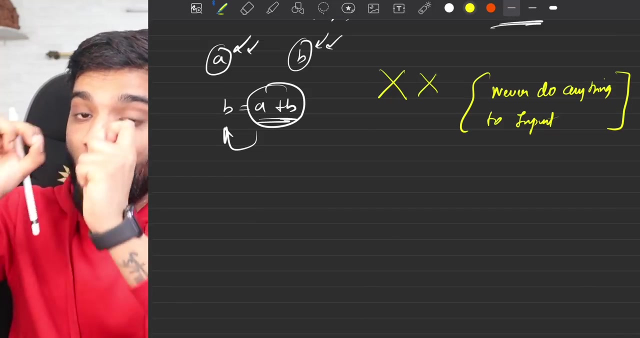 Very, very crucial rule in interviews: Never do anything to the, never do anything to the input, Unless the interviewer Sees anything to the input, because data should not be touched. You can do whatever you wish by taking the data, but you cannot do on the data. 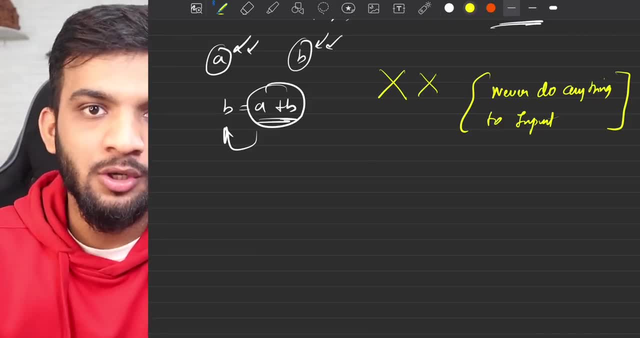 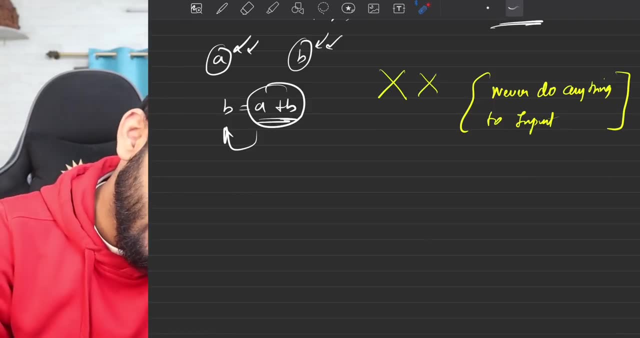 Because if you manipulate the data, it has an issue, because in software engineering that data might be used in some other place. So never ever manipulate data. This might save you a bit of space, but the interview will end up rejecting you, because this is a very, very bad practice. 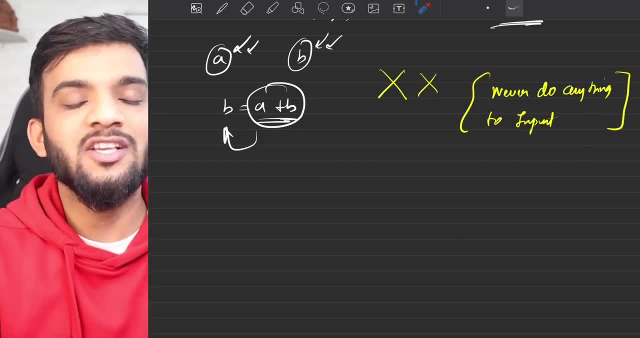 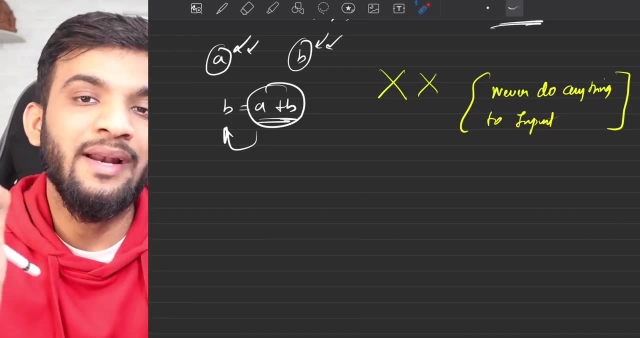 So never, ever, do anything To the input given. always take extra variables, extra array, extra matrix. It might be tempting that if you use the same input variables you will end up taking lesser space, but it's it's not a big concern. 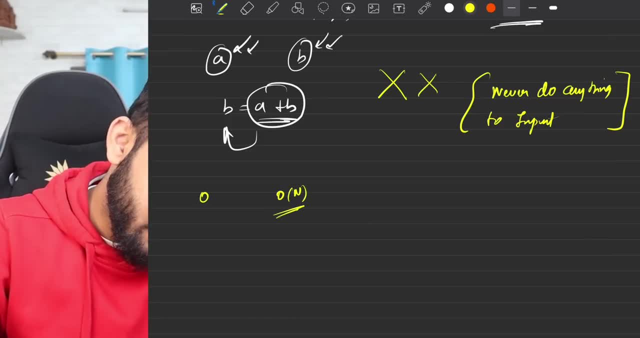 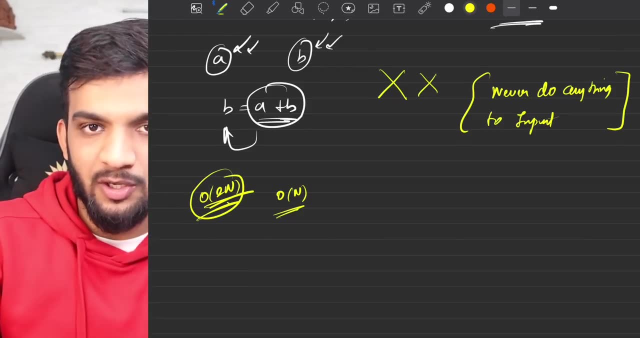 If you're using bigo of n space, like if 2n is used by taking an extra array, it is okay. This is okay. No one is going to reject you if you're using bigo of 2n instead of bigo of n. 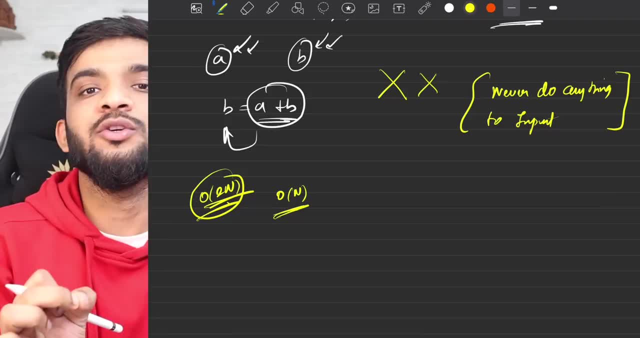 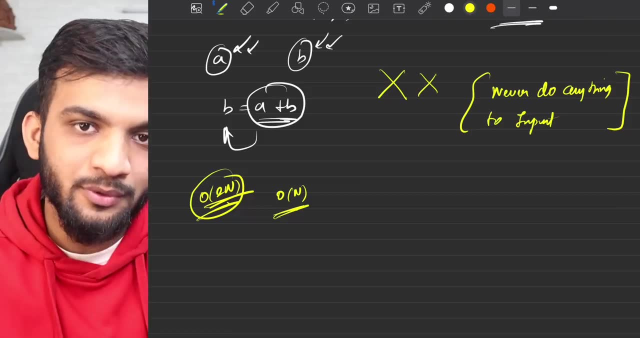 If the interviewer specifically says: do it on the input, Then you can do it. You can use them, otherwise do not, And you can tell that to the interview. You can explain that I do not want to- uh, I do not want to tamper with the data. 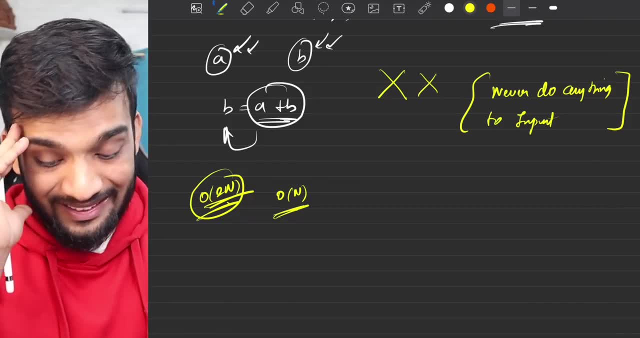 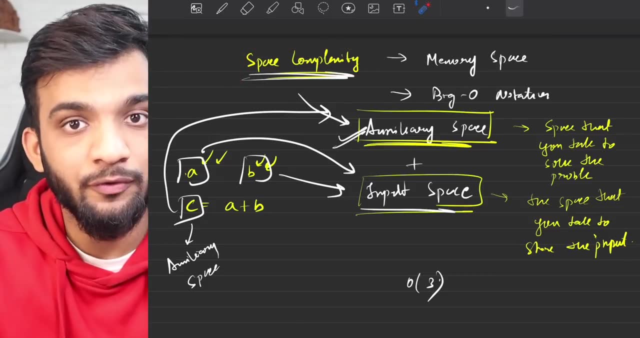 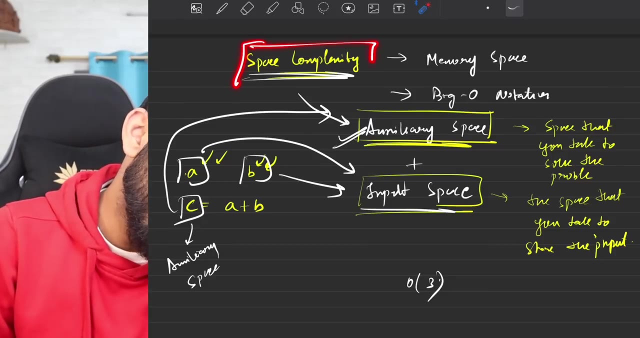 That is why I'm taking an extra variable in order to solve this problem. Keep this in mind for ever. This was about the high level idea about space complexity and the practices you should follow regarding the in-depth knowledge When we solve different problems on different data structures. you will see how I'll be explaining space complexity in depth, because the more 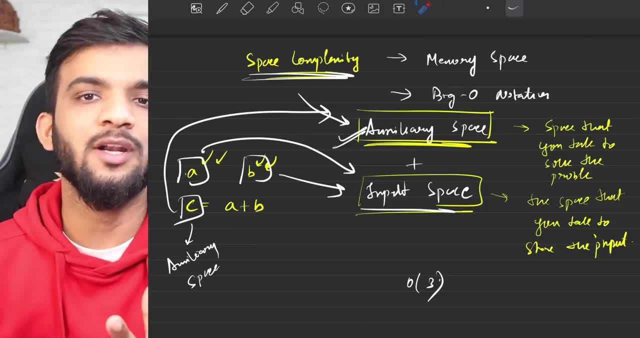 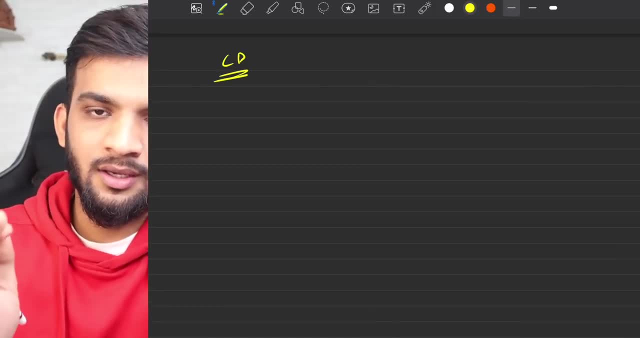 problems. you solve the space complexity. It gets into your head in a much, much better way. So before ending up this lecture, in case you are into competitive programming, then remember one thing over there: you do not run your ports on your Mac book or your windows. 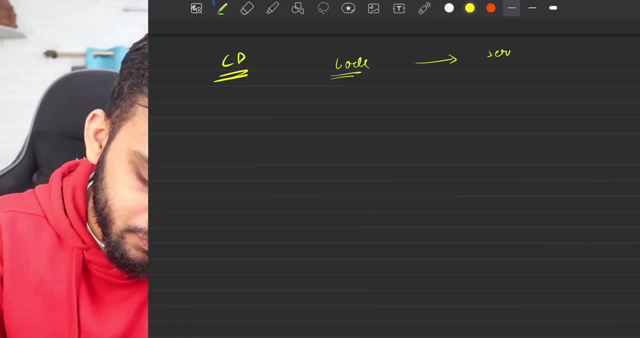 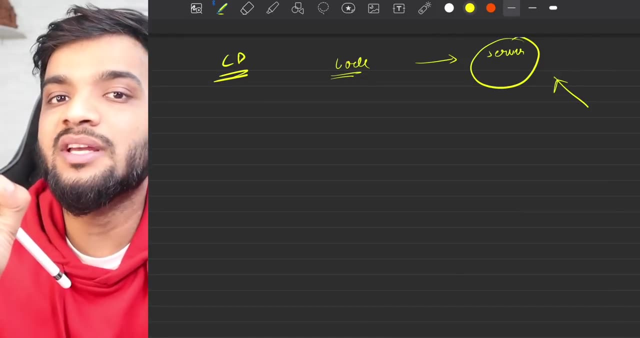 Whatever code you write, you send it to the server. There is a server, you send it to the server. Everyone sends to the same server and these servers in competitive programming- or let's say you're using lead code, or let's say Code Studio- 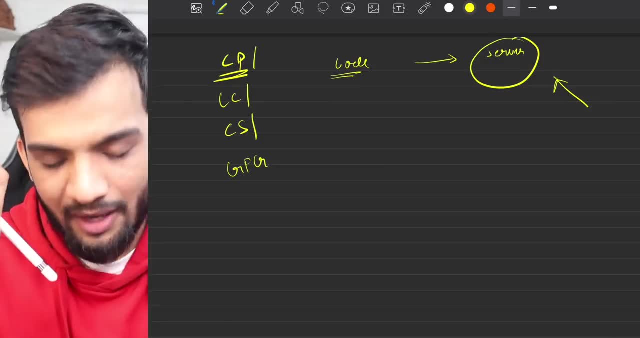 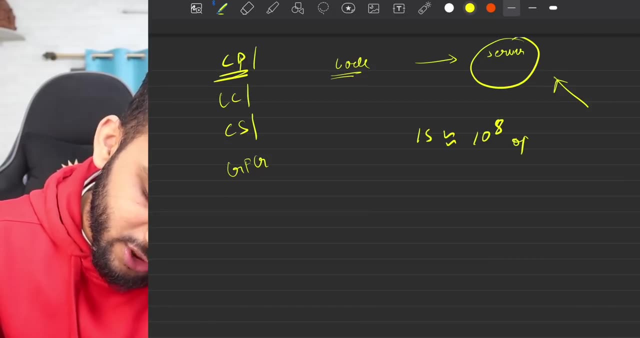 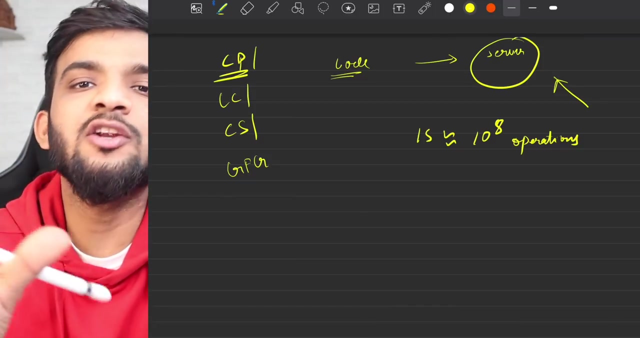 let's say gfg, any platform if you're using. they have their servers and most of the servers take one second for 10 to the power 8 operations. remember this: most of the servers, most of the server, take one second for roughly 10 to the power 8. operation might be 10 to the power 8 plus. 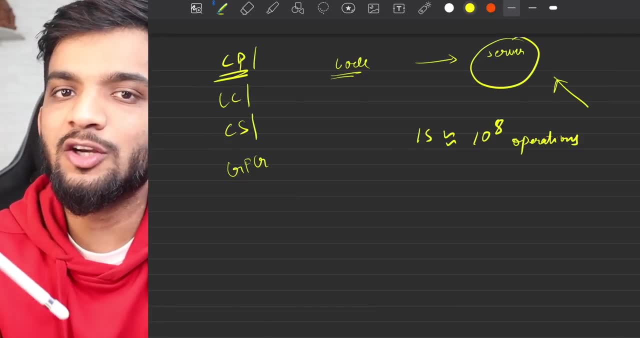 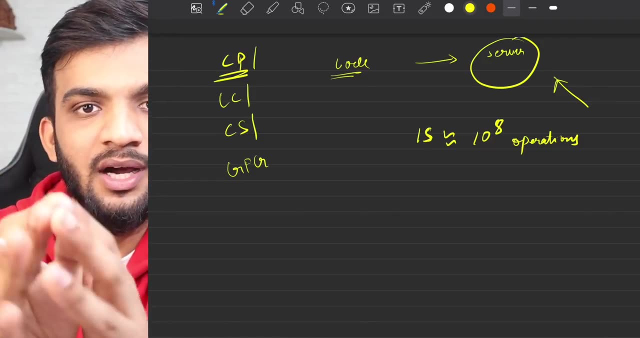 something might be 10 to the power 8 minus something, but roughly it is 10 to the power 8. operations is what you can execute in one seconds on the server. most of the servers are relatively the same and if they're saying two seconds it doesn't mean 10 to the power 16. 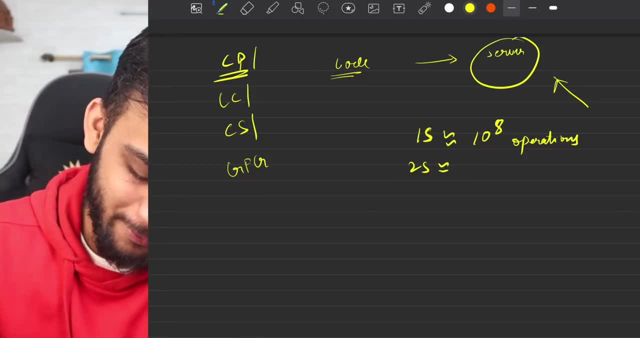 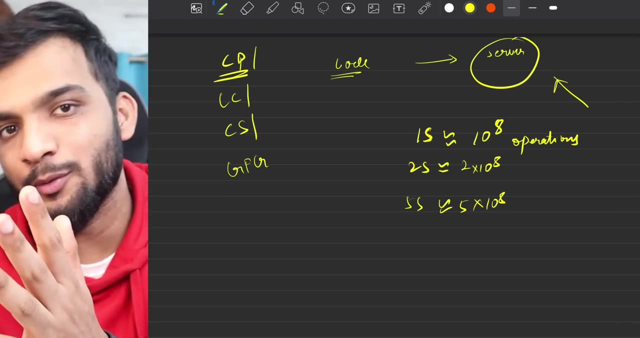 it doesn't. it doesn't. it means 2 into 10 to the power 8 operations. if they're saying 5 seconds, it means 5 into the power 8 operations. do not do 10 to the power, 8 to the power. do not a lot of. 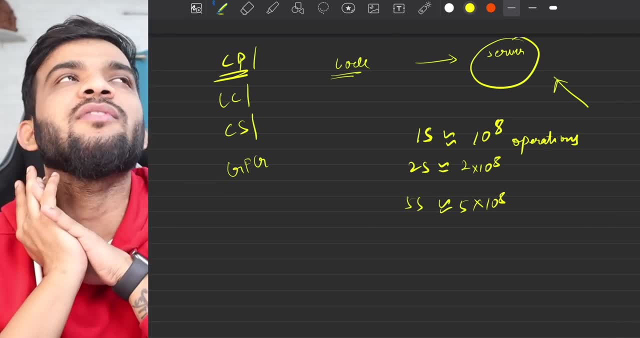 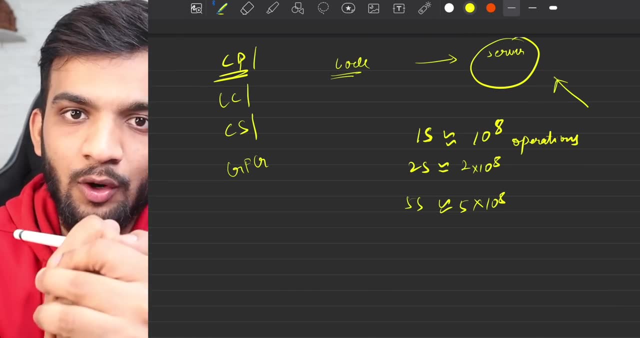 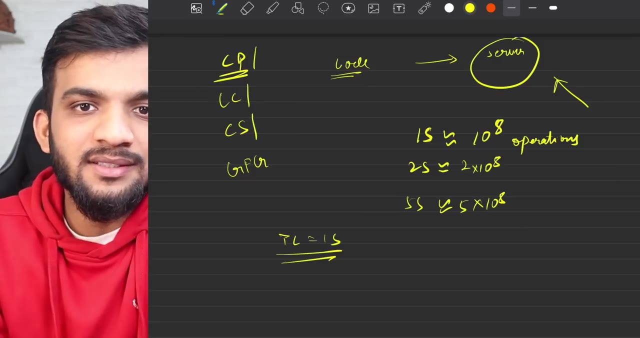 people do that okay. so this is something just keep in your mind, because a lot of times you will see time limit one second. they'll write it. they'll write it in your- uh, let's say, coding round that the time limit given to you is one second, where you should analyze that the time complexity. 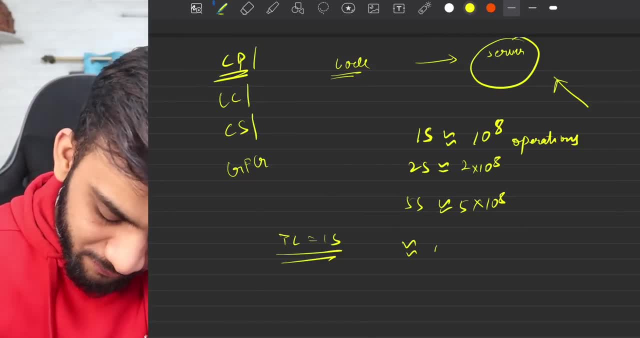 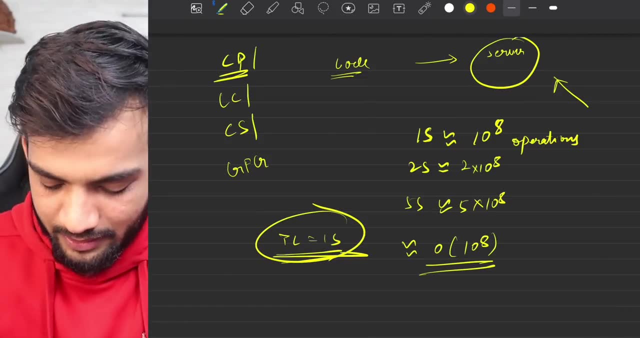 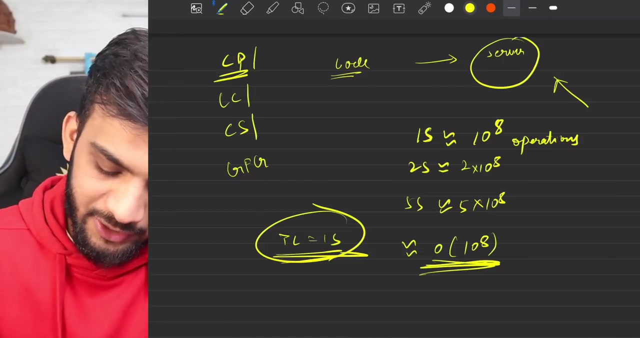 of your snippet of the code or your entire code should be roughly b go of 10 to the power 8 operations. if in a coding round they are stating time limit: one second it means roughly when you compute the time. complexity of your code, avoiding constants, avoiding lower values. it should be b go.